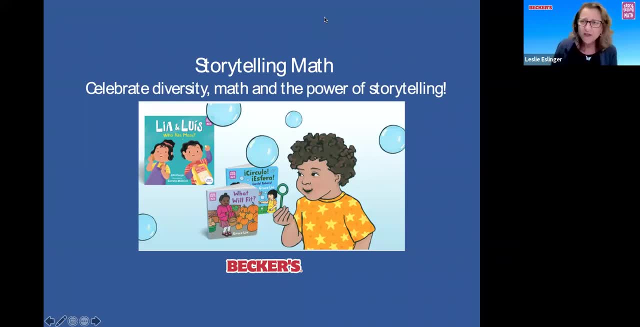 saw one of the authors do a presentation. I knew this was something really special we wanted to bring to all of the people that we work with in the different states- and we have a wide representation. You're going to hear about lots of math concepts, obviously, since we're celebrating. 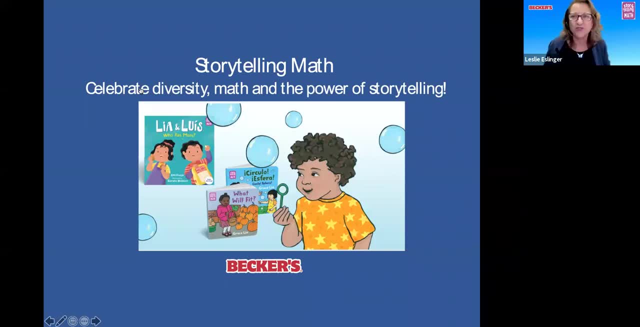 math today and storytelling, But we're also going to see so much in these books about caring, sharing, problem-solving, kindness, a little arguing between siblings, friendship. So so many also social-emotional skills that come out in these books. I think you'll really enjoy them. Let's go to the next. 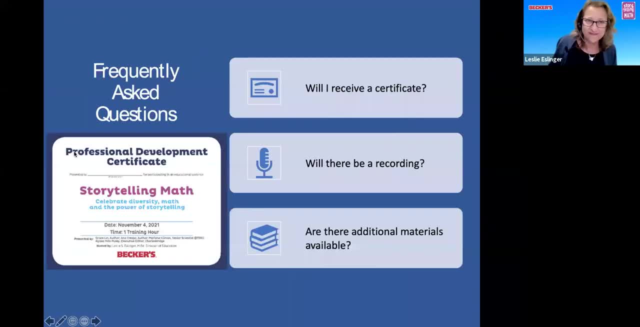 slide. That's a necessary task and the answers to these three questions are yes, yes, yes, You will receive a certificate. There will be a recording available. You will get a certificate in just a moment. I'm just going to go to another slide. You can actually get all that by e-mail. 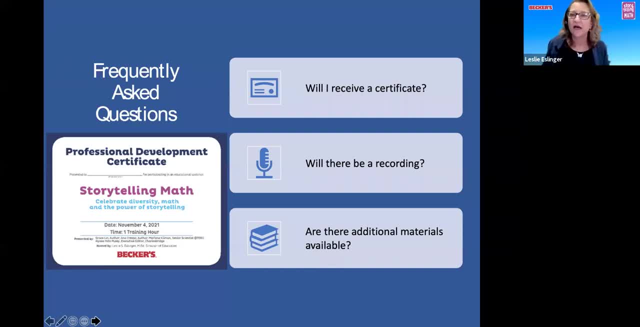 after, within 24 hours after the session, and we have terrific additional resource materials available for you to download. Those links will be placed in the chat box and we will see them at the end, on the ending slides, where you can link to get everything we're going to be talking. 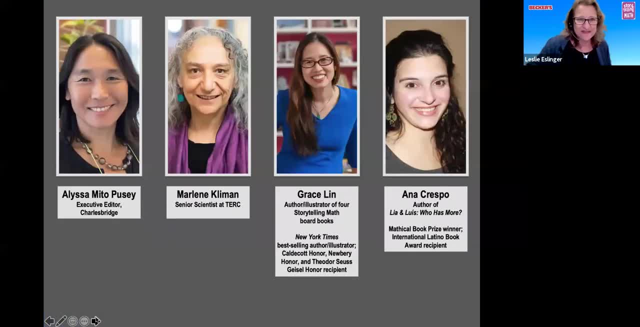 about today and I know you're all looking forward to getting your certificate And if you could go to the next slide, this wonderful opportunity to introduce these terrific people. You can see just by the brief descriptions on screen that we have an esteemed and very accomplished panel of presenters. So 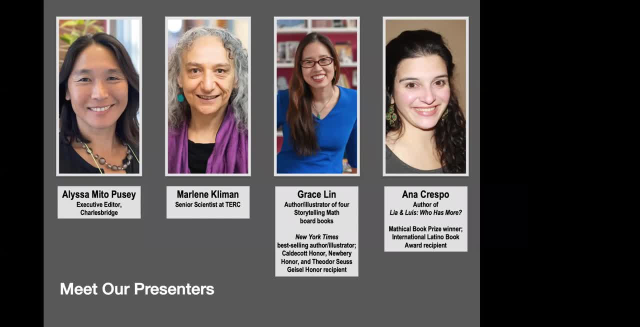 we're going to move from left to right in the order in which they're going to present. First up is Alyssa, and she will briefly introduce storytelling, math books and the Storytelling Math Project. Alyssa is passionate about bringing nonfiction titles to readers that are innovative. 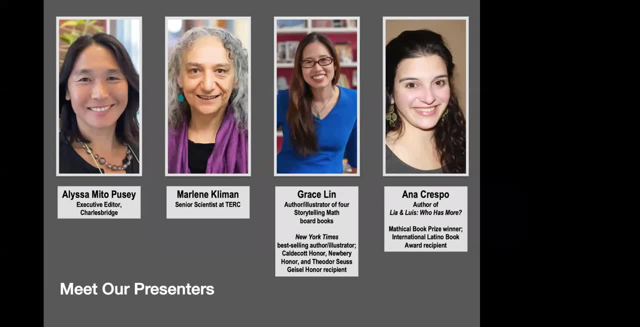 and include authentic, which is really an important word: authentic representation of diversity. Next up, we will hear from Marlene Kleiman. She brings over 25 years of research and development work to projects that focus on mathematics. Not that we're biased in this field. 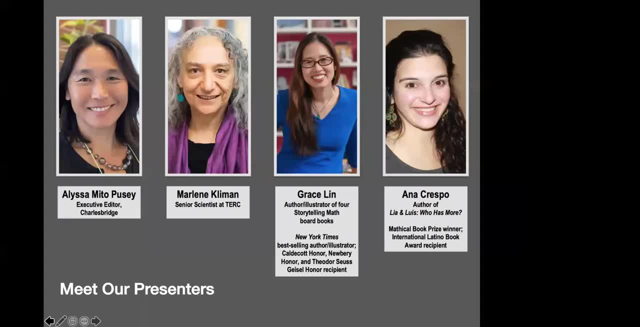 of early childhood, but we're thrilled that she knows how critically important it is to recognize our youngest learners as math thinkers- I love that term. Here Marlene works on the Storytelling Math Project and she's going to be talking about 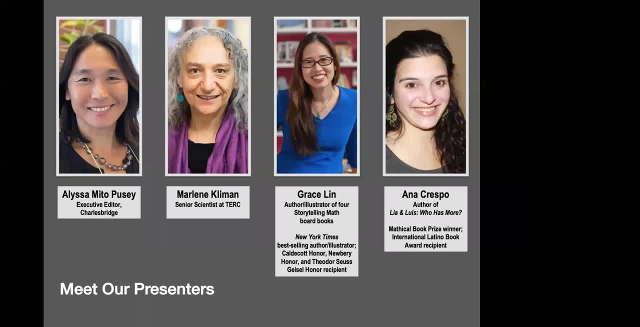 as a consultant for this work, in this case as a consultant for the Storytelling Math Project, and she did some terrific support. We're also so fortunate to have two authors. We have Grace Lynn. Her accomplishments are way too long to fit in this little box here. After I viewed a presentation of 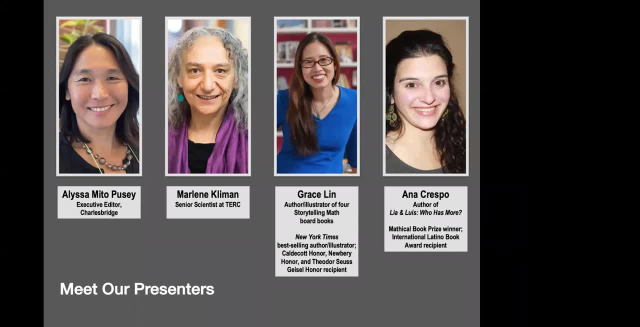 her newest books. I knew you'd all want to meet her firsthand, So we're so excited she can join us. She has a keen understanding of what is important to a young child and how to make a story relatable. We're also excited to have two characters reflective of the children that we teach. 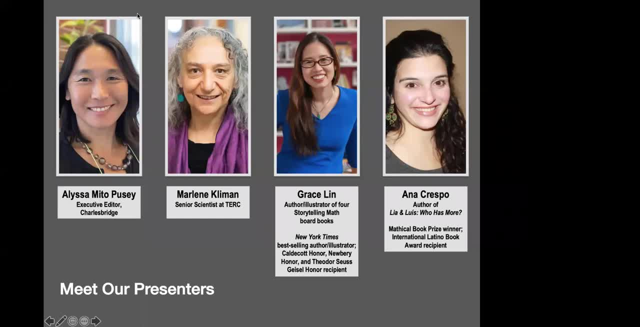 And Anna. Welcome Anna. Anna Crespo, born in Rio de Janeiro, Brazil, She started her career in the field of education and then fell in love with children's books when she began reading to her own children. Similar to Grace's experience, she did not find exactly the cultural diversity she 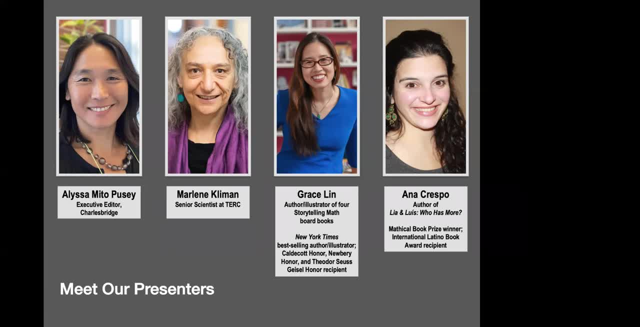 was looking for, so she took up writing with this goal in mind. I hope that's enough to let you know that we have something very special in store for you. Thank you so much for watching. See you next. special in store for you. And now I'm turning it over to Alyssa. 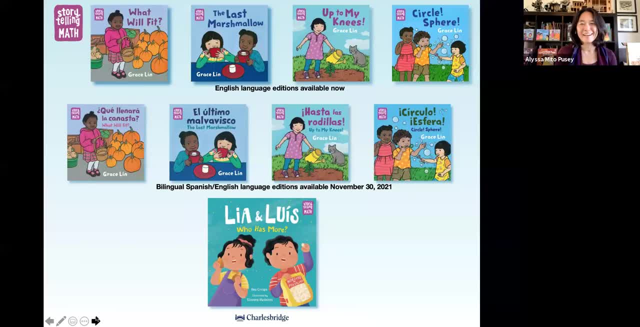 Thanks, Leslie, And thank you everyone for joining us today. Today we're going to be talking about math, diversity and the power of story and how all those elements come together in Storytelling Math- a new series of board books and picture books. You'll get a behind the scenes look at. 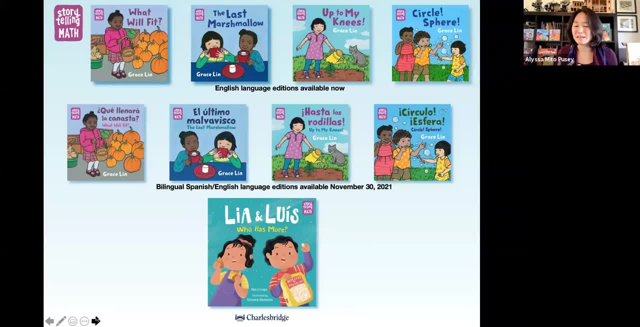 how Grace and Anna develop their stories and learn how to extend the math beyond the books into the classroom and the home. We'll also talk about why diversity is so important in children's math books. So let's start off talking a little bit about Storytelling. Math's mission Marlene. 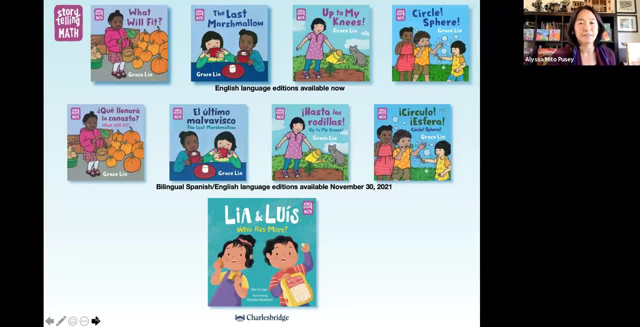 could you please tell us how and why you came up with the idea for the series All right? As early childhood professionals, we know that picture books are a very powerful way to help children make sense of the world around them. But when it comes to picture books intended, 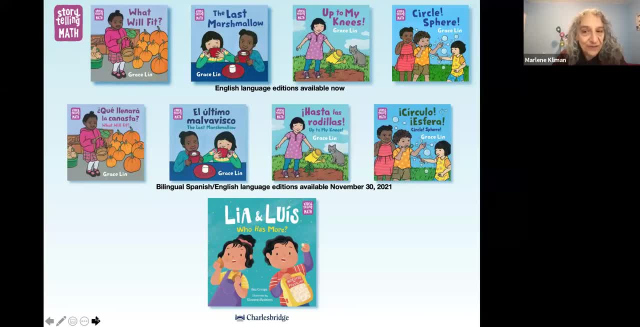 to help children make sense of math. we know that they're not just a way to make sense of the world around them. They're a way to help children make sense of the world around them. So we're going to talk a little bit about Storytelling Math. I've found that there's a dearth of books, with some 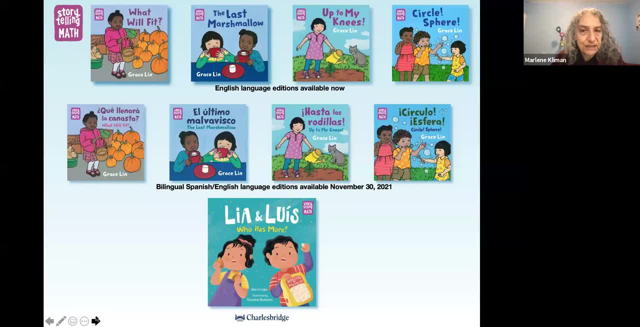 important qualities. A lot of the math picture books in print have animal and white main characters, but few have main characters of color and very few are written by authors of color. Many math picture books center on counting or shapes, but there are other math topics that 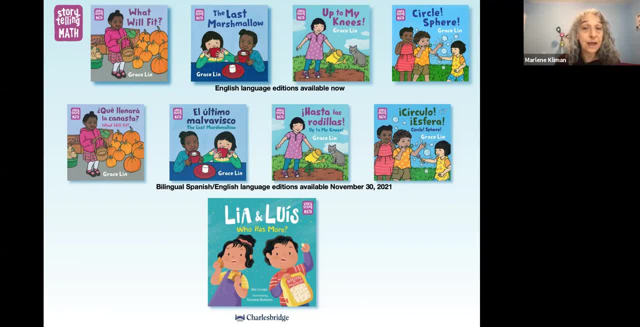 are also important for young children to experience, like sorting, measuring and spatial relationships, And most of the books are more about math than about great stories, with character development and compelling narratives that reflect the social and emotional lives of young children. So Kim Brennaman at the Heisinger Simons Foundation contacted me about helping to develop 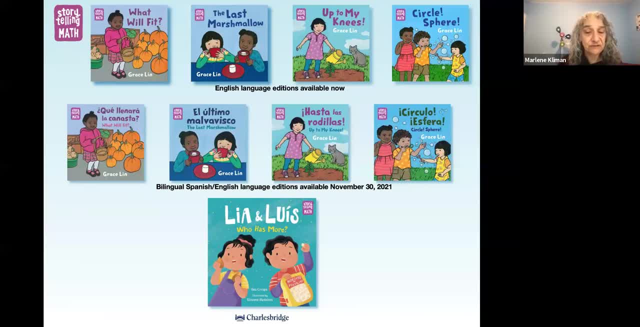 a picture book series that offers a very different vision of what math is, who is a mathematical thinker, who can create math picture books and what a math story can be. So, in turn, I contacted Charles Bridge to work with me on this, Melissa. 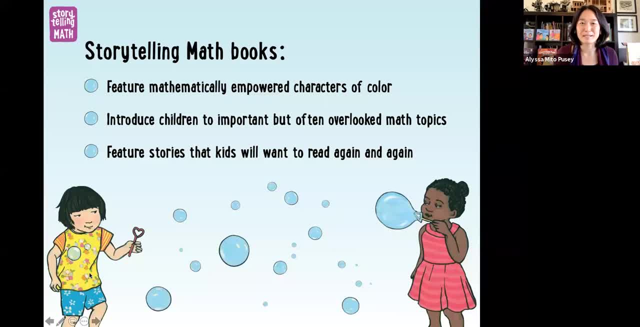 And so we were really excited when Marlene reached out to us because, I mean, here was this fantastic idea for changing the landscape of children's math literature. So Storytelling Math books are different in three key ways. They offer a different vision of what math is and who's a. 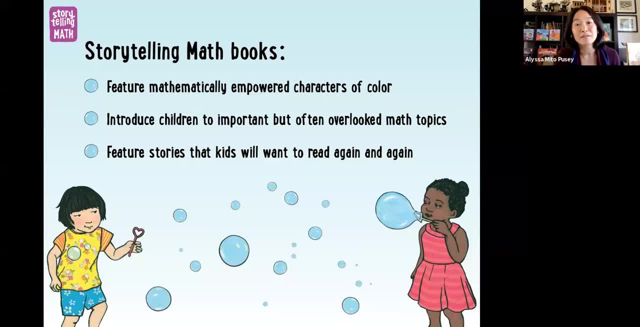 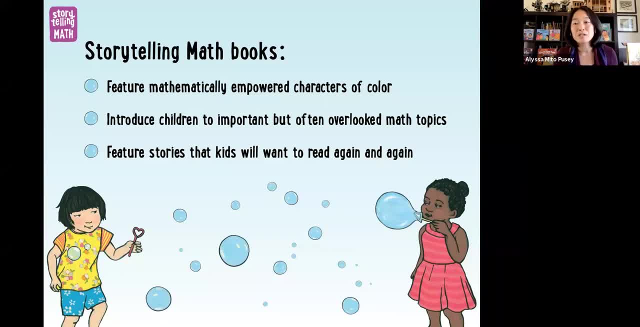 And they feature really compelling, engaging stories that kids want to read again and again. You know we expect in a great picture book characters who care about stories that stick with you and you want to know what happens next. Why not expect the same of math picture books? 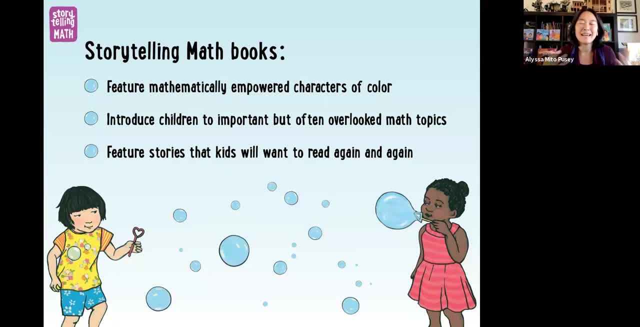 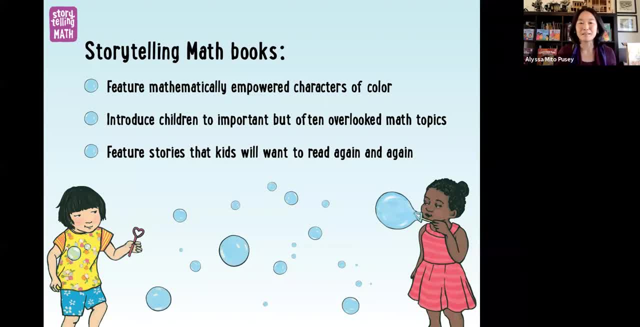 And we're going to do it, And we're going to do it, And we're going to do it. And then we started talking about possible authors And the first name to come up was Grace Lins. So Grace and I had wanted to do board books for a very long time, but we couldn't quite figure. 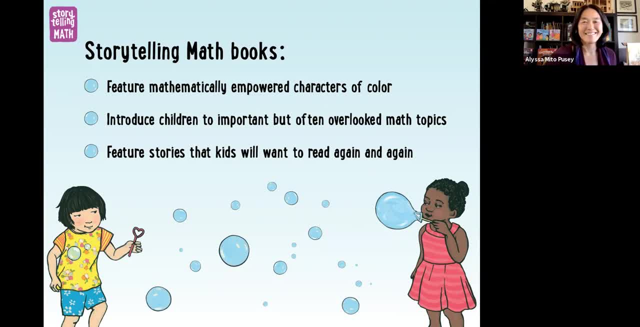 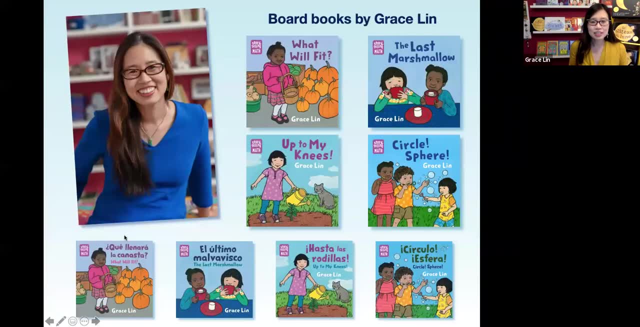 out the right topic. But then, Grace, would you like to tell the story? Sure, If you could go to the next slide. Okay, Hi everybody, I'm Grace Lin. Thanks so much for being here And thanks so much for having me on. 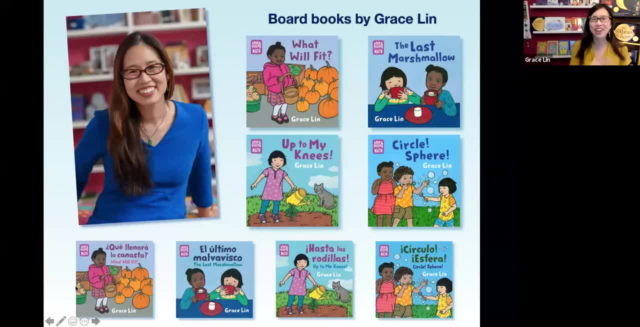 So, as you already know, I'm Grace Lin And I'm the author and illustrator of these board books right here Now. these board books came out last year, But really the seed of these books began probably over nine years ago. Next slide, That's because nine years ago I became a new mom. 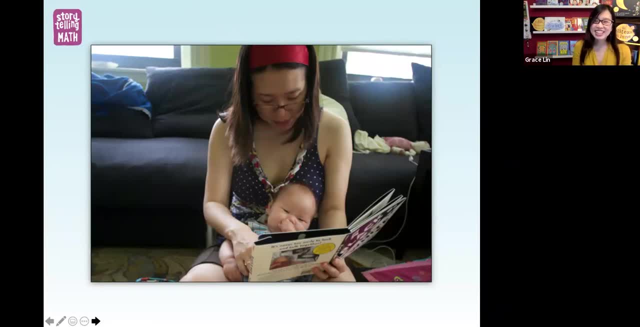 That's me and my baby nine years ago. Looking at that makes me feel really old, Because time has really flied, Flown, flown, flown. Well, anyway, being a very dutiful children's book author, I surrounded my babies with books And I read to her before she was born and after 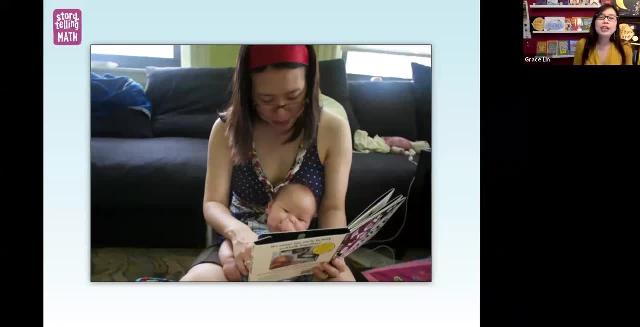 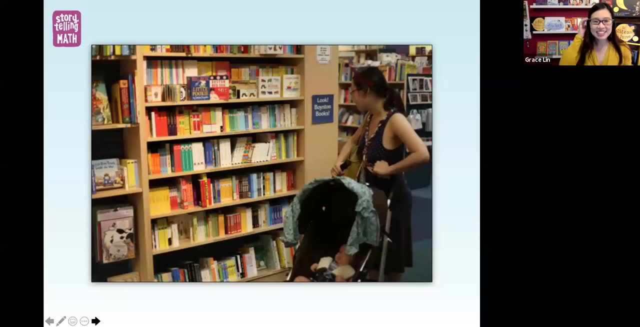 she was born every day, every appropriate moment. I really wanted her life to be infused with books. Next slide, please. But almost immediately I found myself frustrated with the books meant for babies- Very few at the time. Now it's much better now. 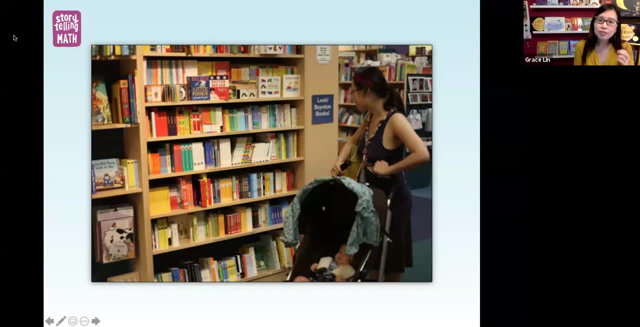 Don't get me wrong, But this is remember. this is nine years ago, So very few featured babies or toddlers of color, Very few featured mothers that look like me or babies that look like my daughter. The very few books that I did find. 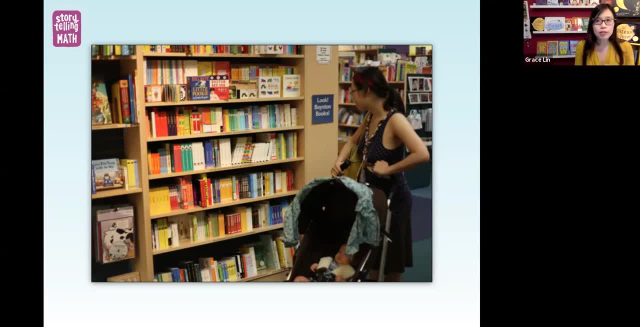 starring babies of color. Most of them were part of the Global Fund for Children series and those are really lovely. If you know anything about baby books. they're really beautiful. They're all photos, But they're all photos of babies from other countries And the thing is that, even though that these books were very lovely, 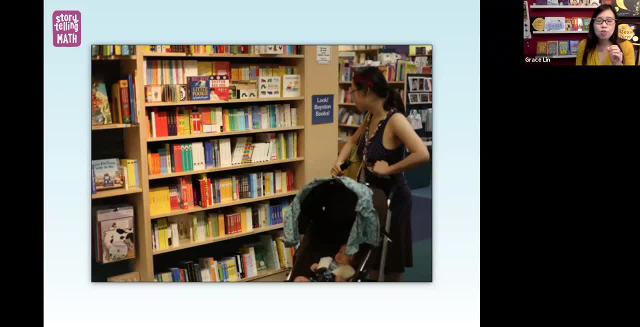 they still kind of gave the impression that non-white babies were kind of slightly exotic. you know they're from other places And they were not commonplace in, you know, mainstream America. So as that kind of- as I saw that over and over again- that kind of planted a deep seed. 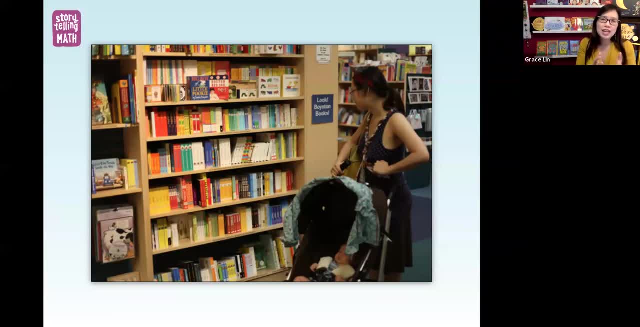 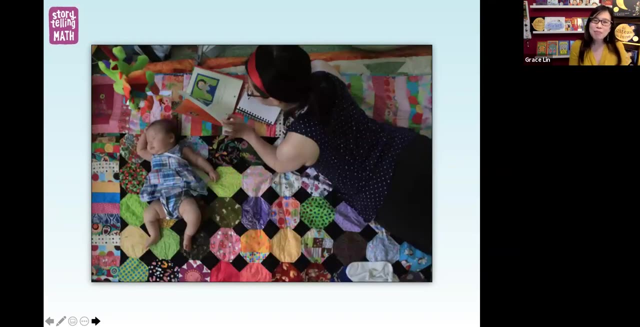 in me to create board books that showed babies of color doing ordinary, everyday things, Babies like my own in Main Street, America, Mainstream. America, Main Street, Mainstream- Next slide, please. So a few years ago I was at an NCTE conference and I ran into Alyssa and I was at 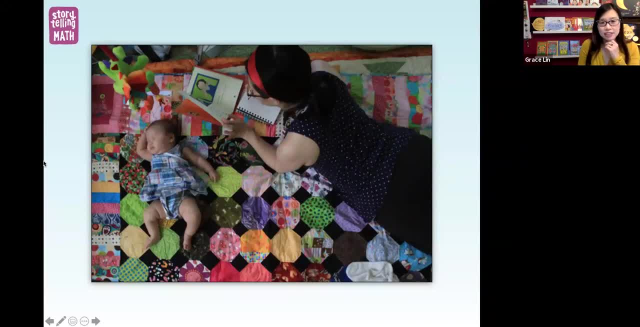 the Charles Bridge booth and I was admiring their Baby Love series because the Baby Love series has a diverse is a diverse series. It has characters of color throughout the series and I was really excited when I saw those And I said, oh my gosh, I'm so happy that you have. 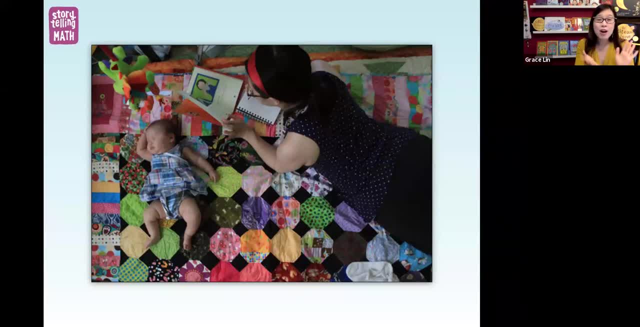 these books with babies of color And I said, oh my gosh, I'm so happy that you have these books with babies of color. And I said, oh my gosh, I'm so happy that you have these books with babies of color, BIPOC babies- because you know, that's really what I wanted when my daughter was. 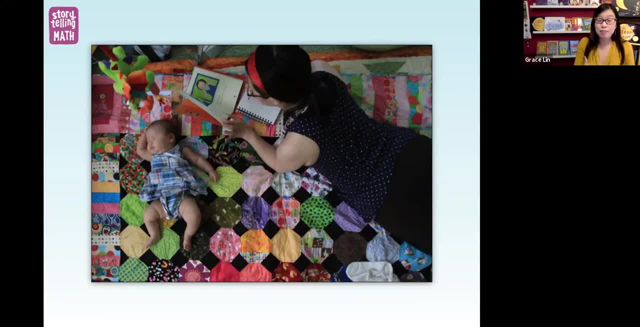 a baby And I really wanted to make, wanted to make these kinds of books too, And Alyssa said, oh well, you should make some with us. And I said okay, And we started talking and we brainstormed a bunch of different ideas, but none of them quite seemed right. And then, a couple years, 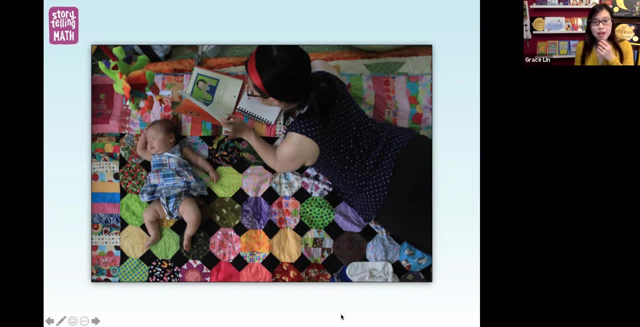 ago Alyssa contacted me because Charles Bridge was teaming up with Turk. I guess Marlene had had approached them at that point- And she said to approach them about the storytelling math series. And Alyssa called me up and she's like: okay, I know that we want to do a board book. 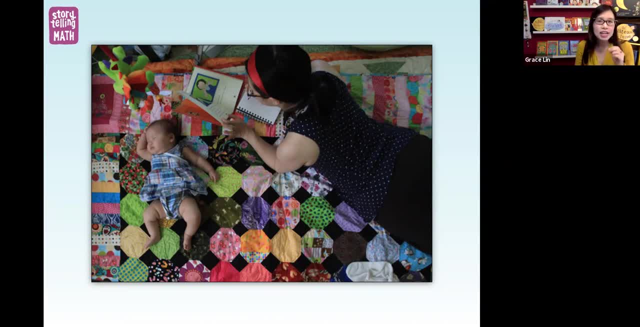 series and you want to do board books. Would you be interested in making math board books? And I kind of hesitated. I said math, you know, like numbers. And she said no, no, no. We want to show that math is much more than numbers. We want to show that math is much more than numbers. 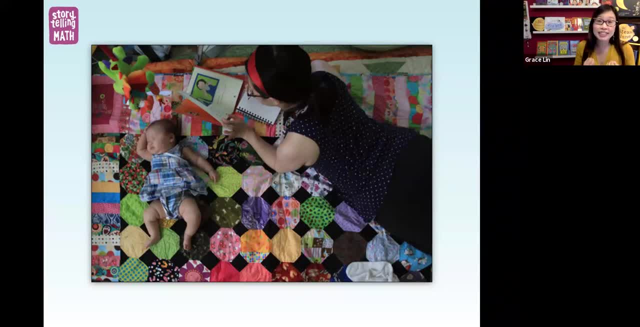 We want to show that math is ordinary and just a part of our everyday lives. And when Alyssa said this, I realized that their ambition with math perfectly aligned with what I wanted to do with diversity in board books And I was like, oh wow, it's the perfect match. Next slide, please. 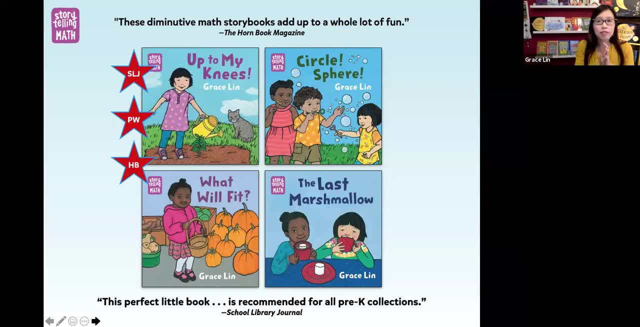 So Alyssa and I decided that a small series of four books, four board books, would probably be the most successful to accomplish our goals. And Alyssa and I both live in New England and we have four seasons here, So it made sense to use the seasons. 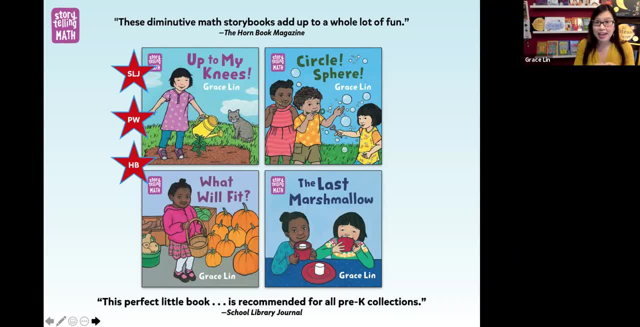 as a framework. So the Asian girl, May, the girl in the series- is based on my own daughter, And Olivia and Manny- the other two characters- are based on her friends, visually as well as personality-wise. I purposely focused each of these four seasons on my own daughter and I. 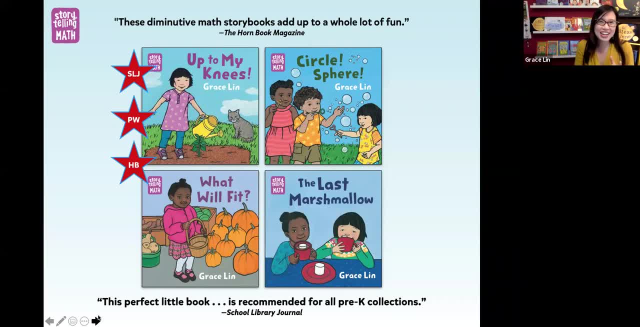 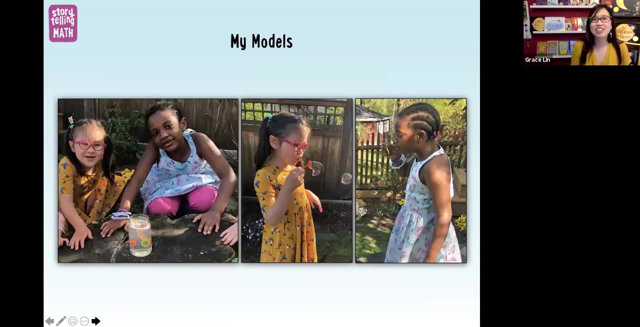 decided to use these books using the everyday fun that she has alone and with her friends, because I wanted to show that these characters and math exist in our everyday lives. Next slide, please. All right, So this is my younger daughter, my daughter, who I used as May, though I used the 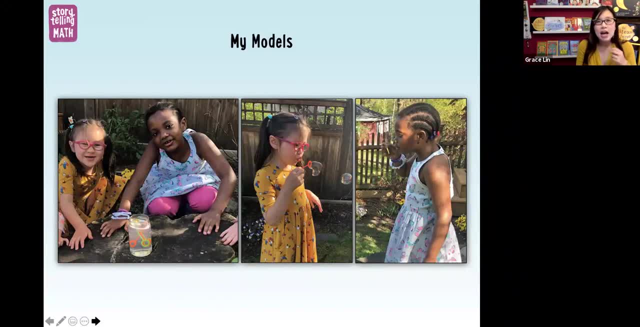 haircut she had when she was much younger, and this is her good friend. this is her good friend as the model for Olivia. Even though the style of illustration that I use for these board books is not very realistic, I felt it was still really important to use models, so these are the models. 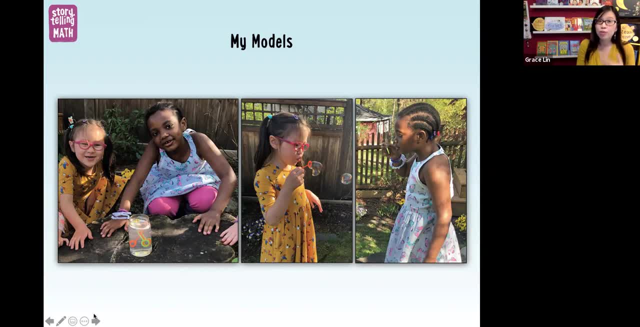 I used For me as an illustrator when I create pictures of children outside of my own race. I feel like photo reference is extremely important, but because without it, it's really easy to accidentally create a racial stereotype, and that is really what I did not want to do. 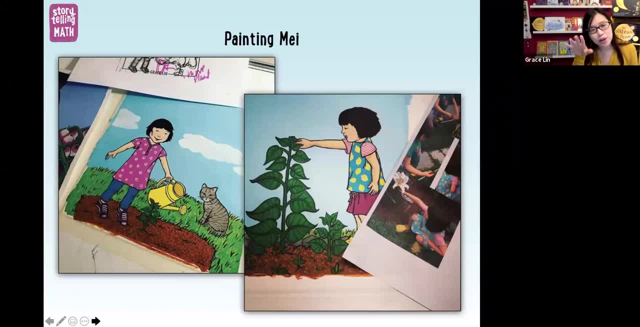 You might see there's a little photo in the right-hand picture. there You can see there's my daughter's old haircut- excuse me, her old haircut- a little bit better. These board books are actually very synchronous with all the things that I've been trying to. 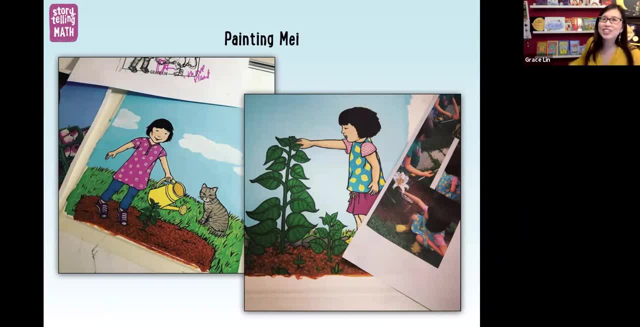 achieve in all of my books. You can see I've been making books for quite a long time and there's things that I've always been trying to achieve. I am a huge proponent and supporter of diverse books, but one of the things I'm eager, so eager- for educators to do. 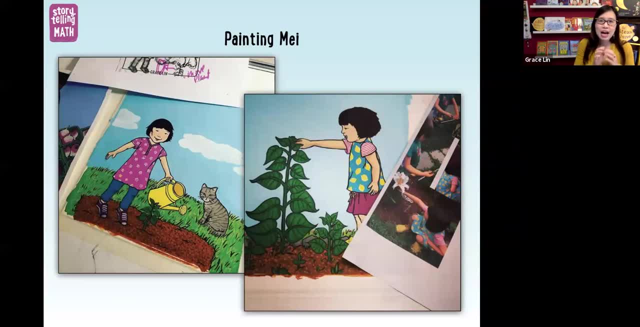 is to kind of unlimit their diverse books. I think there's a misconception that we read books about Asians on Lunar New Year or we read about books about Black people during Black History Month, but the truth is, diversity is every day. Data is the most important resource to us as researchers, and researchers don't. 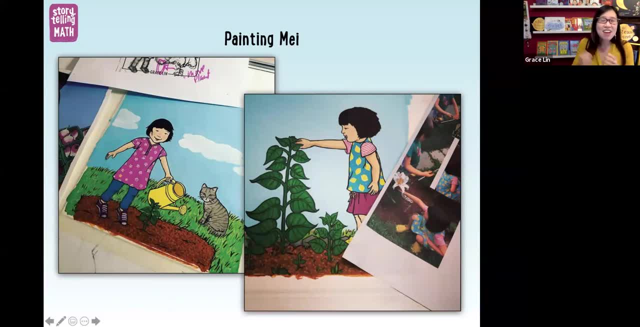 have time to read books about it. It isn't possible, but I think it's important for students to be able to read and think about it, and those are really the key to learning. The other thing I understood deeply about writing books about my family. 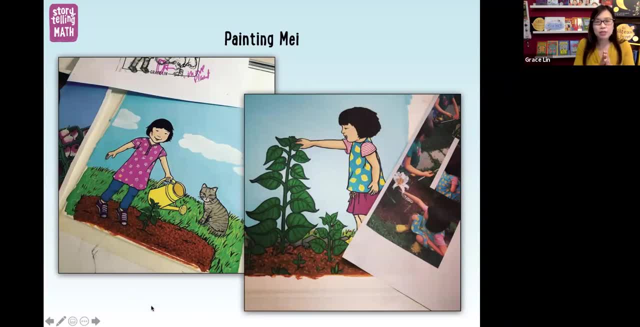 was that it's the same thing with math. I found that I had similar limiting beliefs about math. At first, all I could think about was math is numbers. math is numbers every day, without even knowing it. We use it for sorting, sharing, comparing, finding, even weighting. 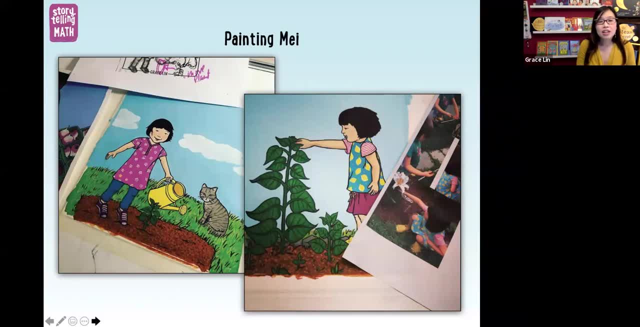 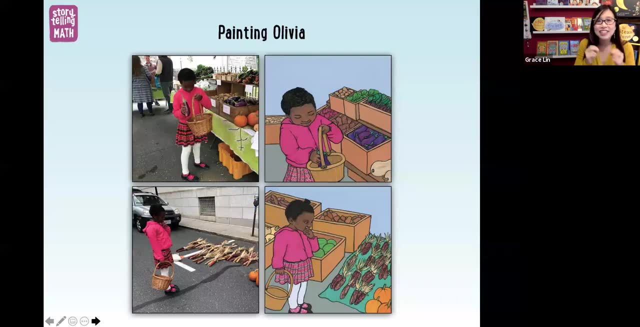 Next slide, please. So math, like diversity, is and should be acknowledged for its everyday existence. But that does not mean that it's boring, And I think what is so wonderful about these books- about all books in general, actually- is how books can acknowledge how extraordinary ordinary things are to a child. 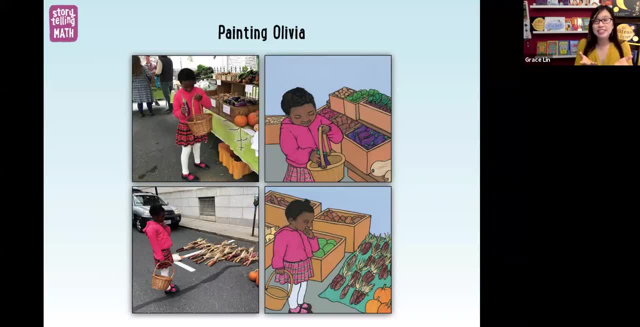 So you know, picking out vegetables at a farmer's market is probably like a really commonplace action to most adults, But to a young child it's a really big deal. To pick something, to purchase is like a momentous action, something that takes a lot of thought. 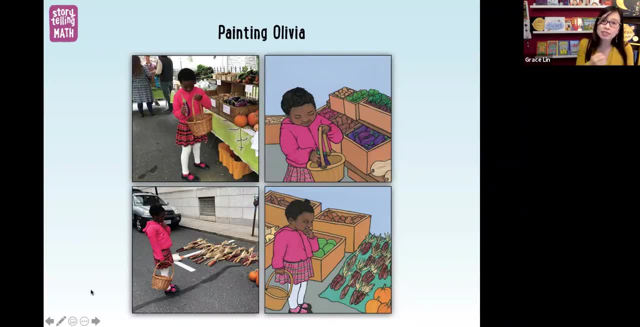 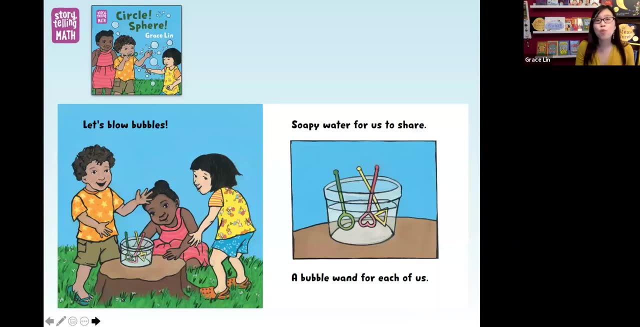 So it's really taking the child's perspective perspective in these books, Next slide, And then in this book, Circle Sphere. it's the wonder of blowing bubbles. You know, as adults we know that when we blow we're going to get a round bubble. 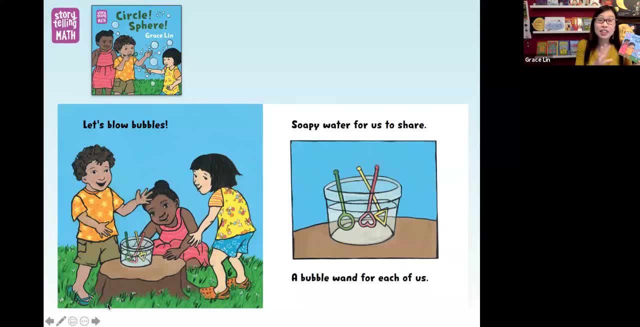 But to a young child this is really unexpected magic with many, many questions. And these board books empower kids by recognizing the exceptional nature of these simple events while being interwoven with exceptional, unique experiences of diversity and math. So I'm going to read you just a couple of pages of this book, which I hope kind of illustrates what I mean. 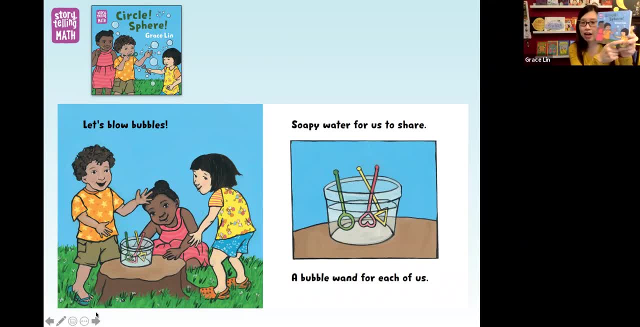 OK, so this is Circle Sphere, And just so you know that this is the, this is May, the one based on my daughter. This is Olivia, based on her friend, And this is Manny, another character that is based on her friend, Another friend of hers. All right, 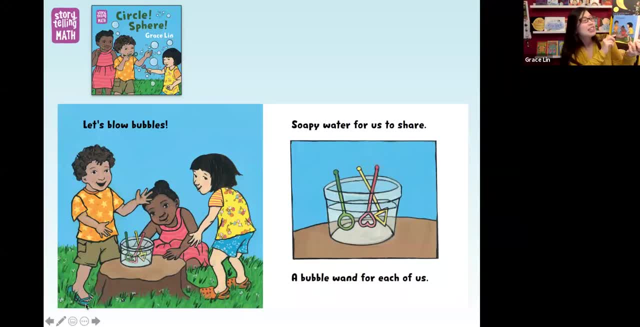 Oops, Yes, OK, we're on this page. Let's blow bubbles- Soapy water for us to share, A bubble wand for each of us. So here you have three friends. They're about to blow bubbles. You can see the soapy wand and also already see a little bit of a hint that these wands are different. 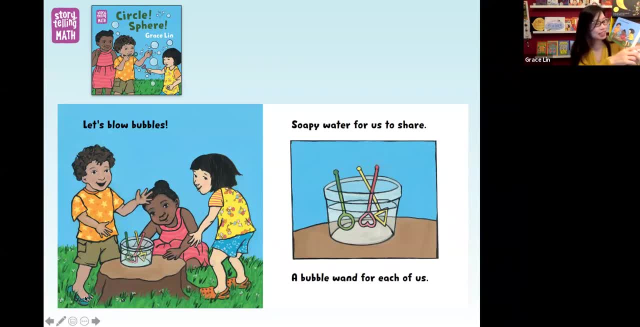 They all, they're all going to be used to blow bubbles, but they're each different. And you know, in a way, that's a kind of a nod to these friends that they're great friends But they're all a little different. you know, visually, OK, next slide. 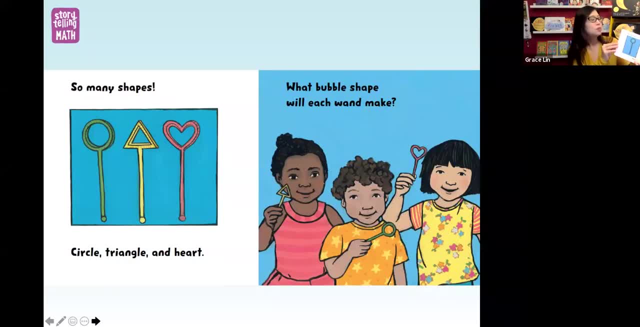 These pages are stuck. Sorry, my page got stuck. There we go So many shapes: circle, triangle and heart. What bubble shape will each wand make? So you know, like I said, this is kind of taking this very simple action of blowing bubbles and showing how there really is so much wonder and mystery to a small child about that. 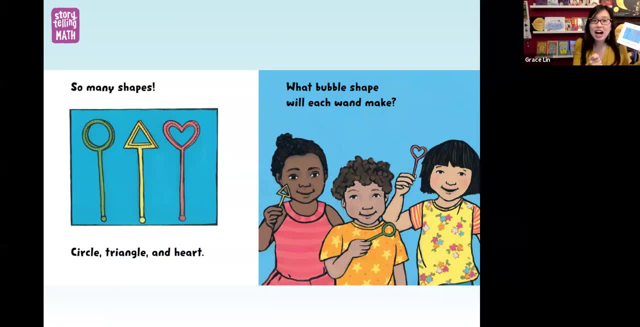 You know, when a child gets a triangle wand, you know the first. there's always something in their head Like what shape will blow out. Will I get a triangle bubble, you know, or will I even get a bubble at all? 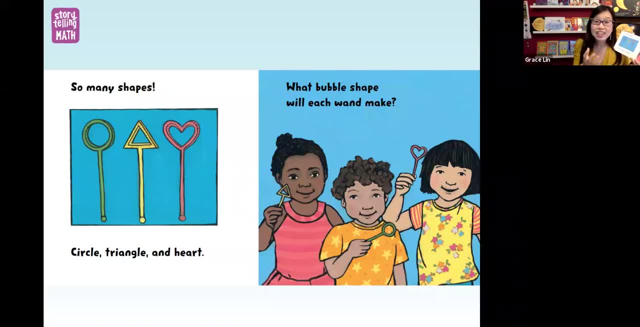 So these are all things that are really, really interesting. Or you know the idea that these are flat and the fact when you blow it, it will create something 3D, which is something that Marlene will talk about next in the activity that goes along with this book. 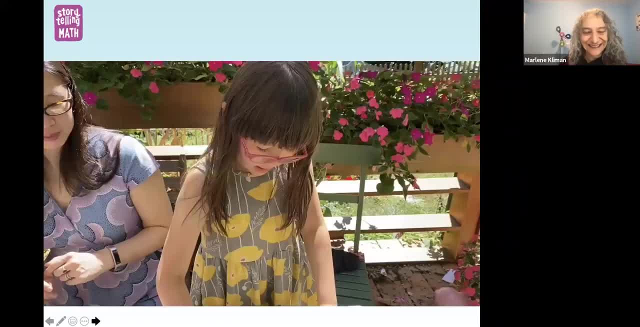 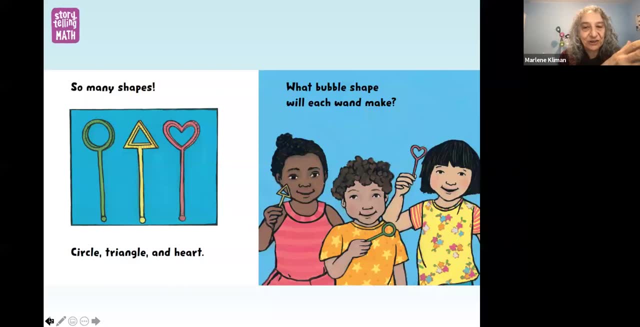 So, Marlene, come on up. OK. so, as Grace said, the story takes the everyday experience of blowing bubbles and highlights the inherent opportunities for children to engage with math ideas like round, flat, spherical, 2D and 3D. 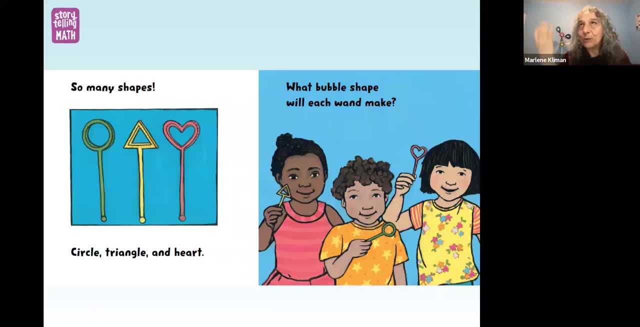 We say math is all around us, but if we attended to it it would be a very different world. So this helps you attend to it. And, anyway, each storytelling math book comes with math information and some activities at the back of the book. 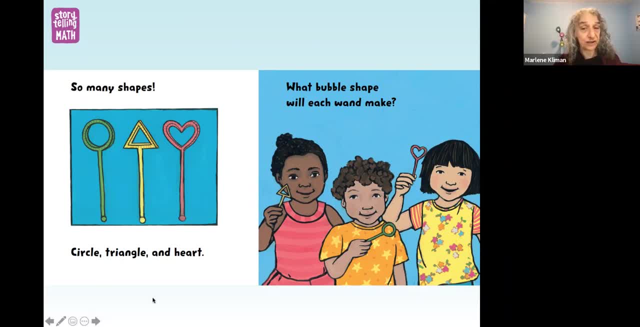 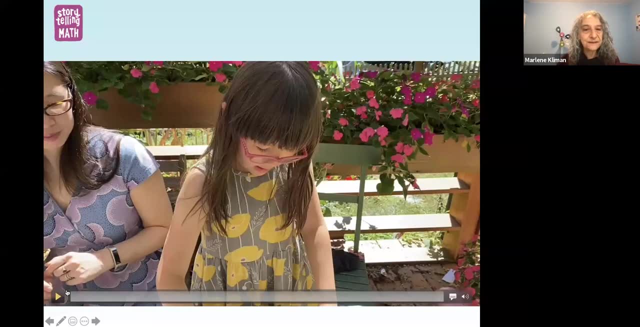 And it's free downloads, And Grace is going to show you one of the activities that further explores relationships between 2D and 3D shapes. So with bubbles we go from you know flat to big and round, And here we go in the opposite direction. 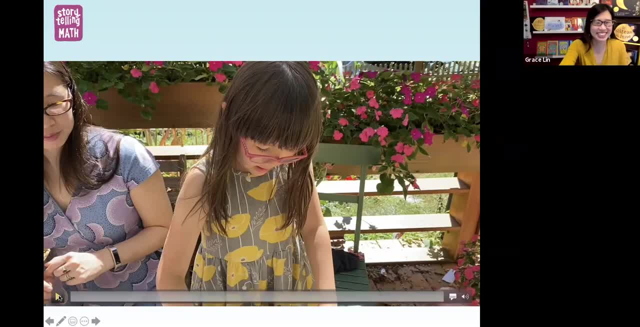 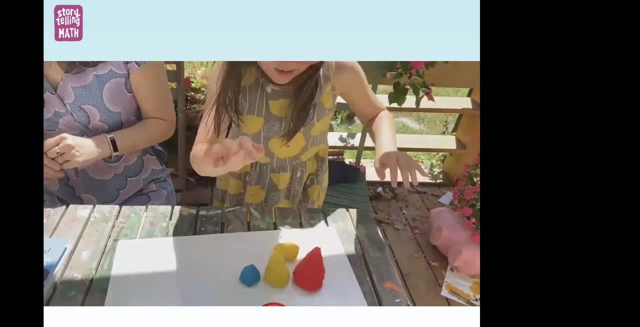 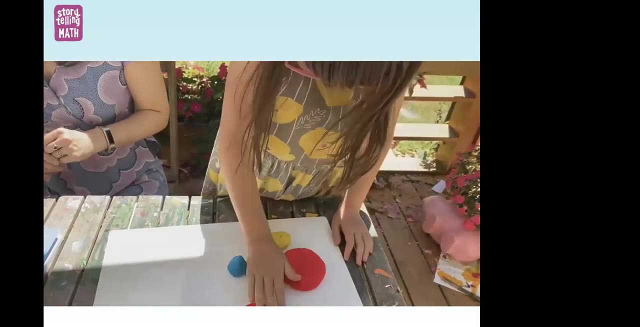 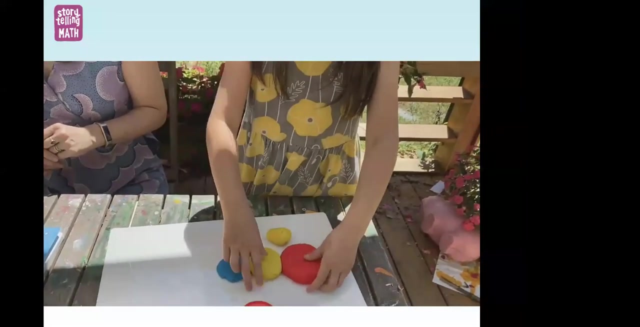 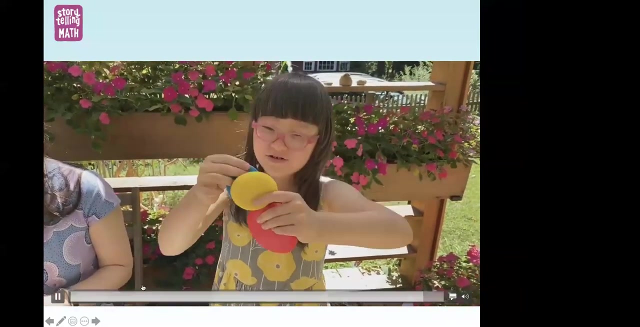 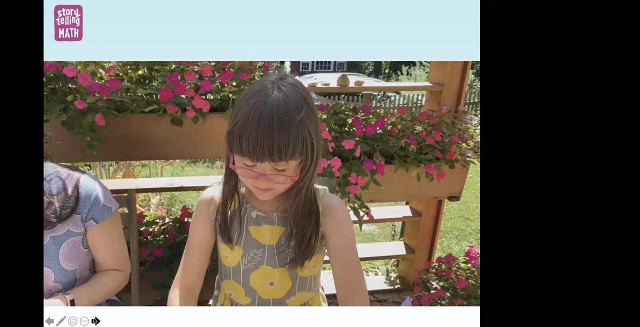 Time for the video. This is my daughter, by the way. I made three different cones- They're all cones, Wow- And each one made what shape? A circle. Yay, All of them made the circle. So I think we're going to the next slide. 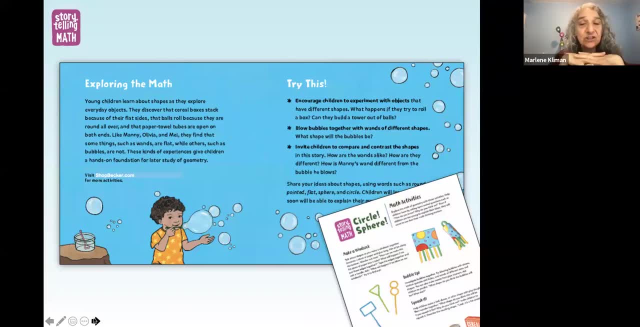 Yes, OK. So the activity Grace just showed- Squash It, or a little piece of the activity- promotes learning in a very tactile and physical way, which is an important way to learn math at all ages. As children do the activity, they start building a bank of concrete experiences with shapes. 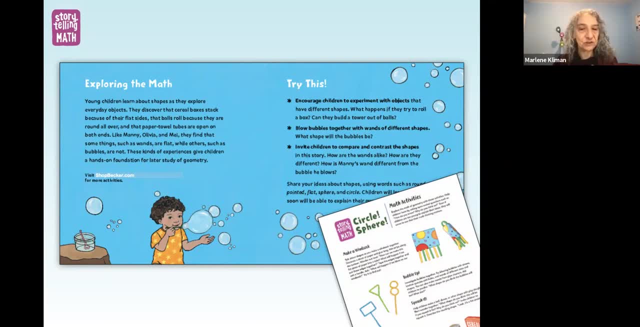 That will help them make sense of geometry when they study it in school. in a more abstract way, The activity can offer a math experience, you know, creating shapes with Play-Doh and then squashing them to children of a wide age range. Babies and toddlers can participate and experience that transition from big and round to flat by just squashing. 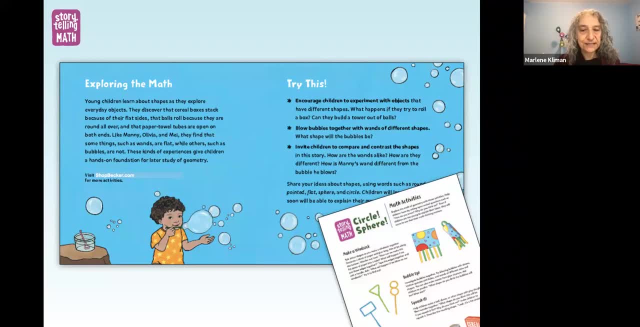 But young school-aged children, like the ones that Grace was with, can also talk about the process. They can predict, as you saw, they can reflect and that way they can deepen their understanding. So Grace does the activity with just a few kids, but you can do it one-on-one or with a larger group, whether you're at home, in a library or in a childcare program or in a classroom. 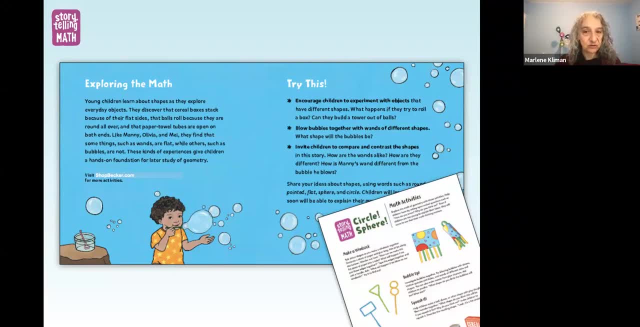 So, as you see here, at the back of each of our storytelling math books there's an explanation of the math written by a leading math education expert, Activities that extend the math And some of the activities. And some of the activities are available as free downloads. 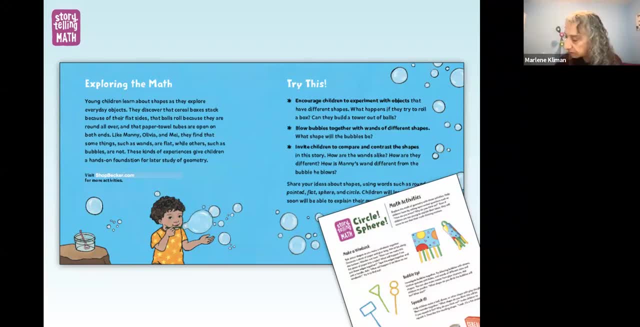 So any more about the math from anyone. I just want to say that these activities are really really wonderful And so much of realizing how, of taking what I was saying about the extraordinary, the ordinary making the ordinary extraordinary, is really just paying attention. 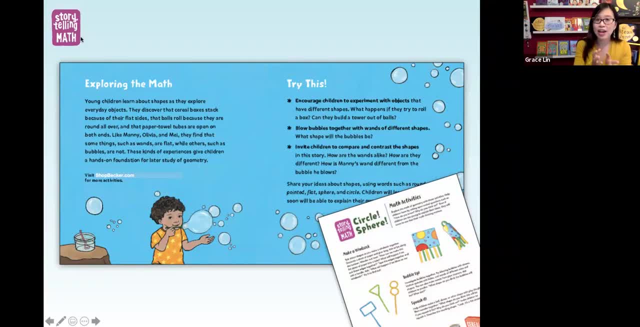 And doing these activities is just a way to help you pay attention to the math in your life And I think that once you start doing it, you're going to be able to do it. And I think that once you start doing them- like you saw, I did with my daughter- like you start seeing it everywhere, like all these different things- 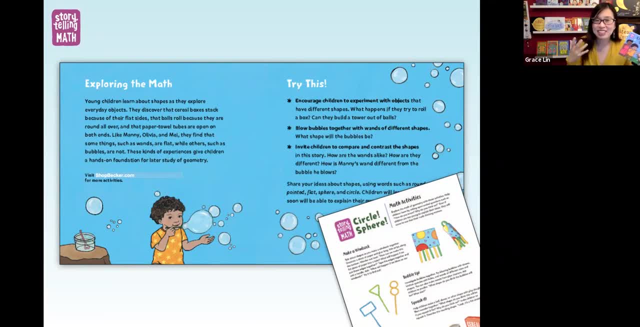 And it's really a really kind of magical thing to experience life with like a whole new, different lens in a way. And I'm going to jump on too, because one of the things I loved in the last marshmallow was the point that was made in the activity section about fair does not always mean equal. 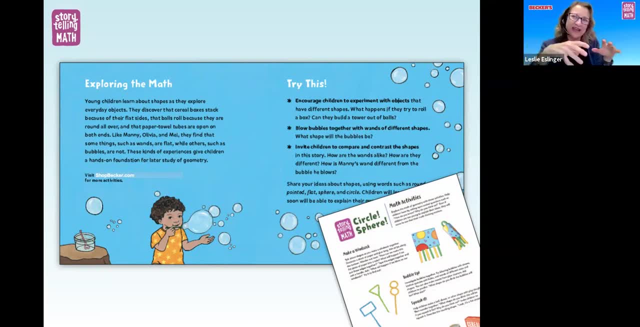 And I thought that was just such a great concept. And I thought that was just such a great concept. So, as you can see again, it's not just the math concepts, but so many good social concepts are coming out of this as well. 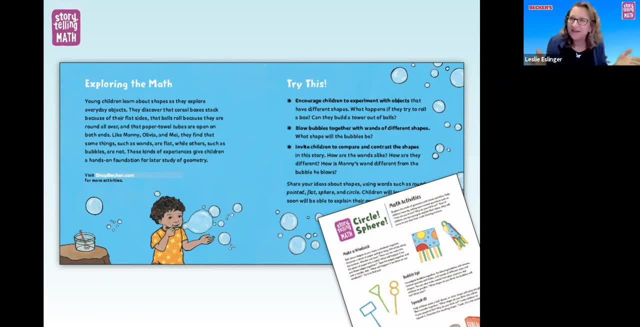 And obviously, with our new understanding of equity, fair does not always mean equal, And I just think it's a great concept. So make sure, when you do get these books, look at these books, to really pay attention to the added information at the end. 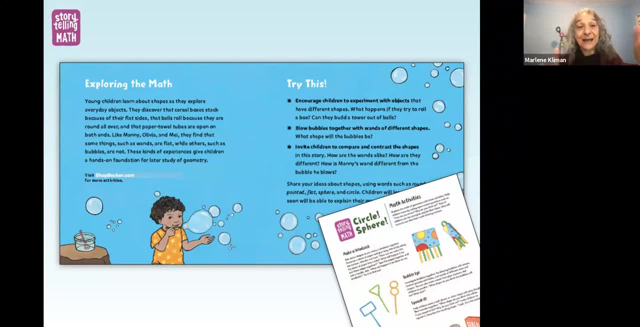 It's really insightful. Now, just to add to that, in that particular book there are two kids sharing three marshmallows And they're trying to figure out how to do it, And Grace just did an amazing job on their facial expressions. 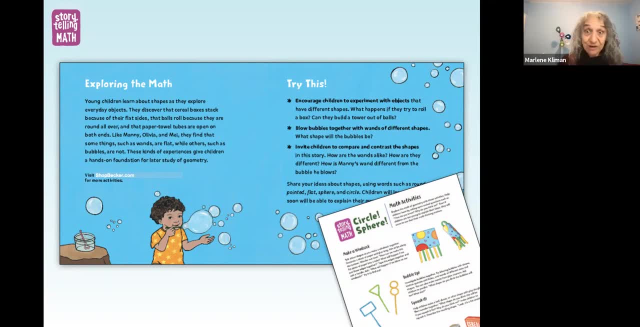 And they're angry. Who is going to get that marshmallow? Can we find a way to share it? And there's just so much emotion. If this were a word problem, then you would know what to do. You would have everyone get one and a half. 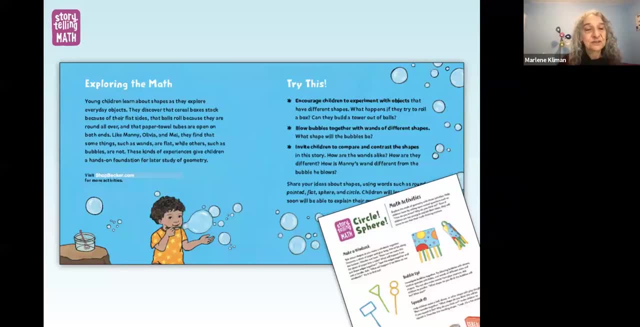 Story is done Over, But there is a lot more in life than finding a mathematical solution, And I think that's a really good point. Math might be part of the solution, but there's emotions too. I just wanted to add one more thing about math being the solution. 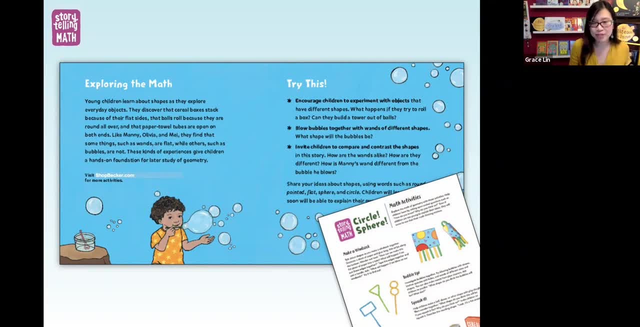 Because I think that is really, really important that I kind of want to reemphasize, especially for the last marshmallow. It's the idea that we have two kids here. Whoops, I'm going to. All my pages are stuck together. 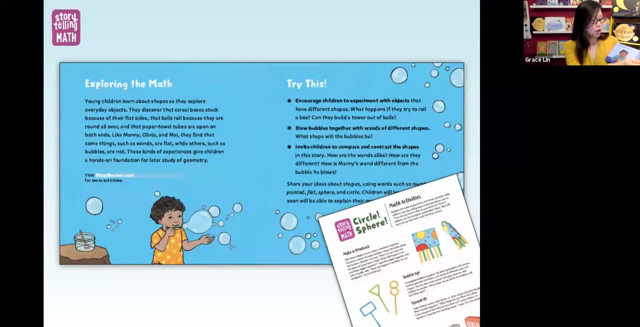 So we have two kids here who, Who basically have a problem and they have to kind of solve it themselves, And what's, what's lovely is that they use math to solve their problem, And I think that's the whole message that we're trying to set. 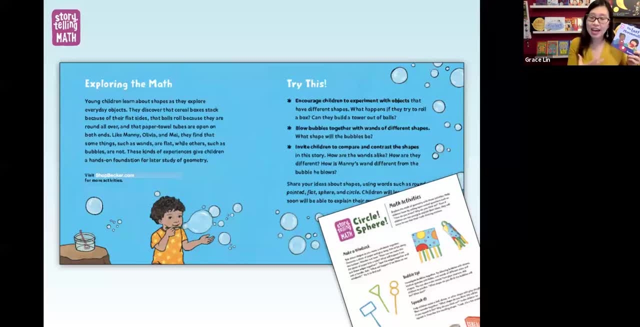 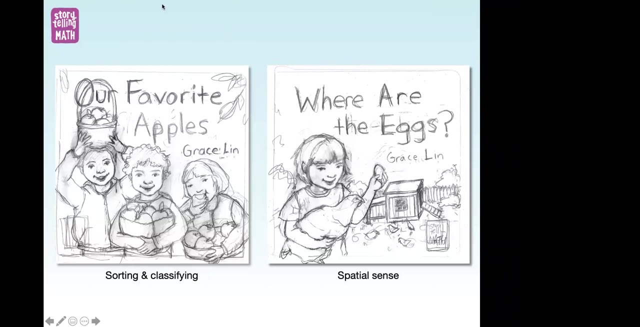 Send to young readers is that math can help you find the solution, and many times is the solution, And I think that's the whole message that we're trying to set, And I think that's the whole message that we're trying to set, And I think that's the whole message that we're trying to set. 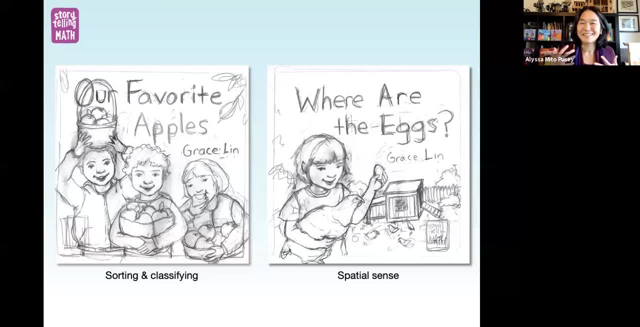 Okay Yeah, The stories are really great, Featuring empowered kids solving their own problems, And they're going to keep on Finding math in their everyday life. We're going to give a little sneak peek Into what's next for Olivia, may and Manny. 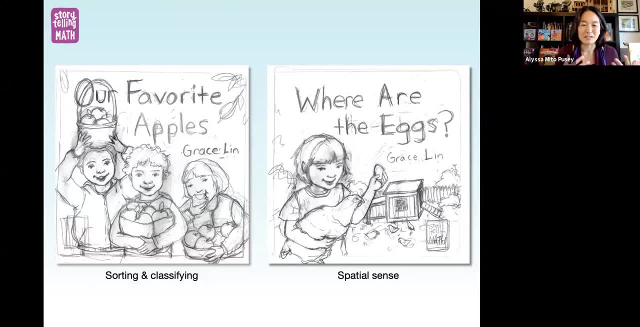 Grace is working on the next four board books. We one is our favorite apples. Which star Which starts all three kids. It's called The Where are the eggs? stars may, And it's about spatial sense. And there are two other books also coming, one about patterns and one about 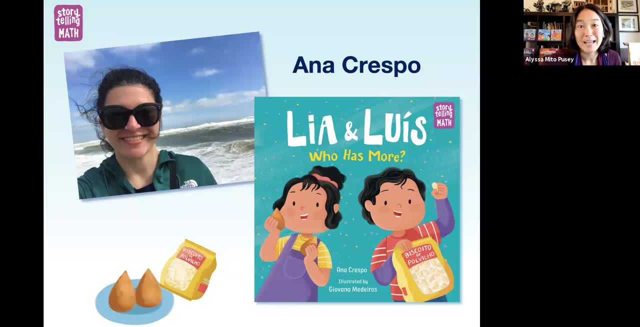 number sense. So I just love these cover sketches and I can't wait to see all of the sketches grace. So, as we mentioned, Storytelling math includes both board books and picture books. more than 500 submissions by some very talented authors. It was a real challenge to choose the 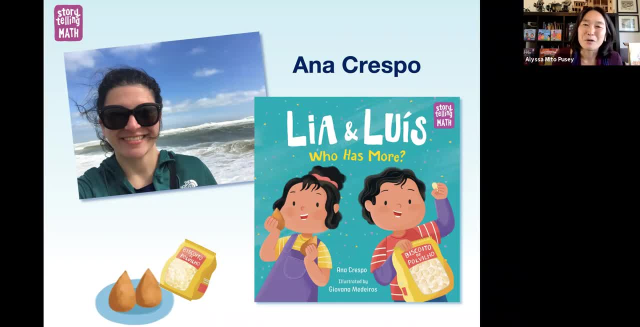 best of the best, but the very first story we chose was a no-brainer: Leah and Luis. Who Has More? by Anna Krespo. We immediately fell in love with Anna's charming characters, playful writing and seemingly effortless incorporation of math. And the story came about because of a chance. 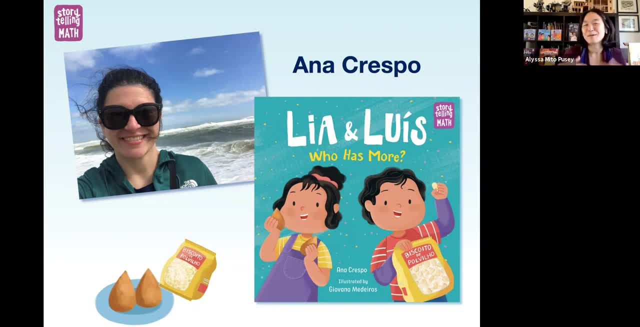 encounter. Could you tell us, give us a behind-the-scenes look at the book Anna Sure? Hi everyone, Thank you so much for joining us today. I am Anna Krespo, the author of a few books, including Leah and Luis, Who Has More, and of the sequel as well that is coming out next year. 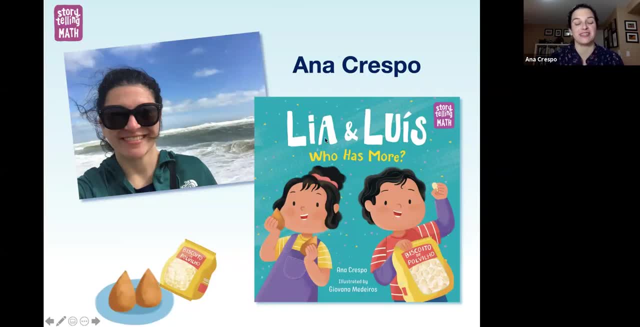 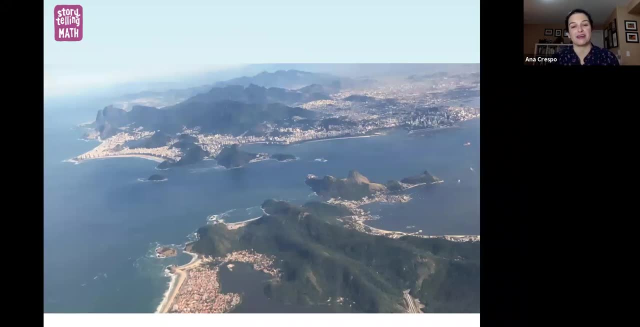 But let me talk about this. Leah and Luis, if you can change to the next slide, Alyssa, please. So I was born and raised in the beautiful city of Rio de Janeiro, Brazil, and I currently live in Colorado, the foothills of the Rocky Mountains, where I love. 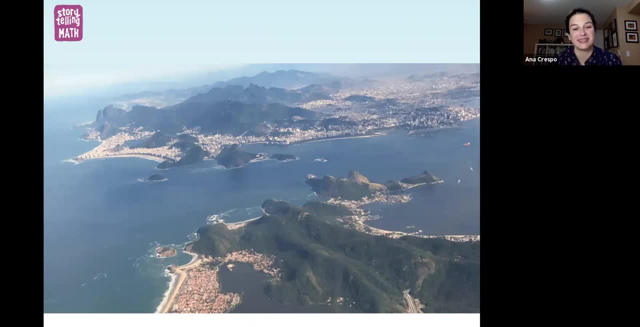 all the trees and the forest and everything, but I very much miss the ocean. I did meet Alyssa by accident during the Public Library Association Conference which was in Denver. I don't remember the year exactly, but I think maybe it was 2018.. Not sure. So I met Alyssa and she did mention. 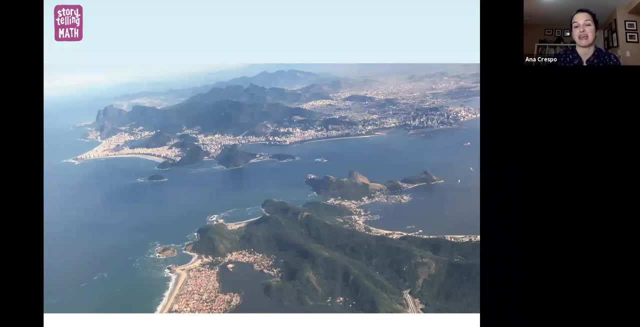 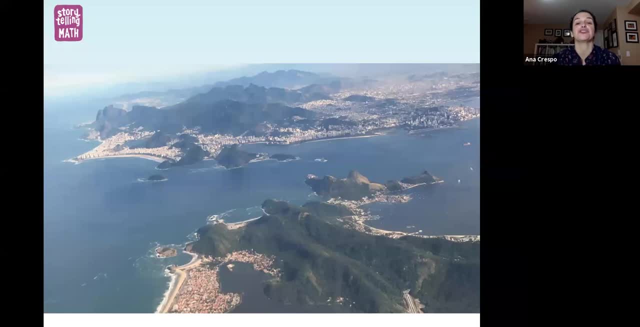 but it was a series by diverse authors featuring diverse characters in mathematical plots, And so she asked me if she could send me the file with the details of the series, and I said yes, sure, But only because authors are usually like, really looking forward for opportunities to. 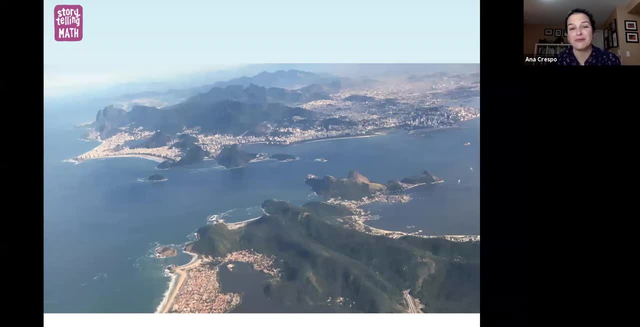 connect with editors. I really didn't think that I would be able to write that And so anyway. so Alyssa sent me the document and I continued to think that I wouldn't be able to write the book, just because I had never written a book based on a prompt before. 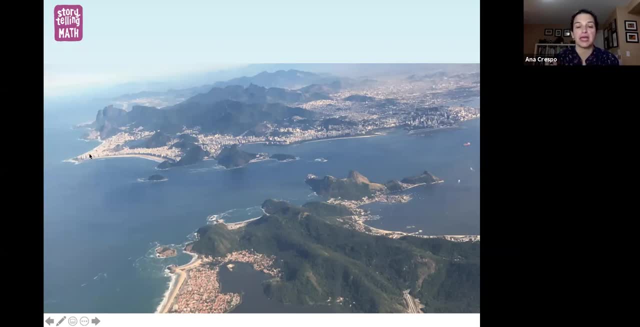 So it was very new to me And part of the problem that I had was that I kept thinking about the math and the math and the math, and I was focusing on the math, But really the idea was to have a book. 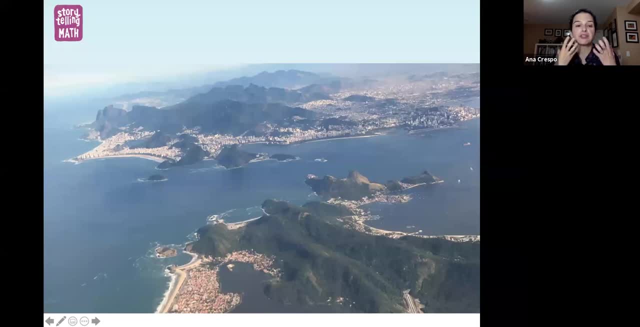 um, a story. right, the idea was to have a story that would flow really, really well and have a plot that was based on math. actually, can we keep, yes, the real just for a little once, a little while? um so anyway, um. so then, what I had to do was that I had to, um, stop thinking. 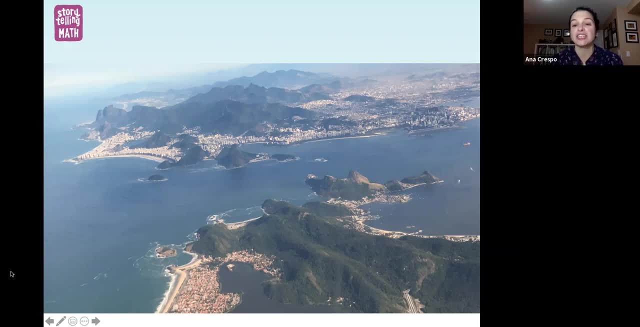 about the math and you start thinking about my childhood and my culture, and it was really like a memory exercise. I tried to remember the games that I played with my friends, the routines, my time at school, and I finally remembered this one question that my parents used to ask me. 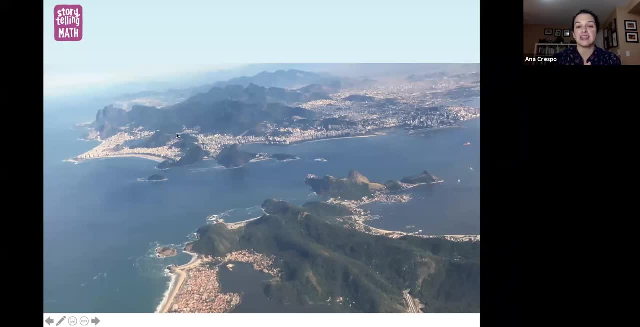 what weighs more, a kilo of lead or a kilo of cotton- and I do understand that this sounds like more uh, uh, Americans likely um, because you know what kid knows what lead is. but uh, in Brazil we use the word shumble, which means lead, to refer to very heavy things, and so, even if a kid doesn't, 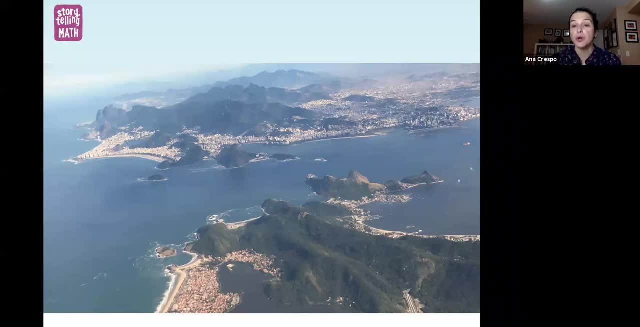 know what lead is, the kid will know that lead is very, very heavy- it's like an expression, almost- and so, of course, one kilo of lead and one kilo of cotton. both were effective, and that is exactly what I was thinking about. the point you said about how 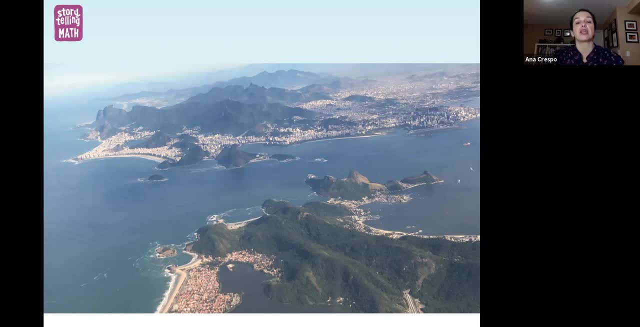 lead is a very, very, very heavy, and of course we haven't been told about it in much detail. but so weigh the same. but a kilo of cotton will occupy a lot more space than a kilo of lead, And that's really how the premise for Lee and Louise came about. And now the next slide, please. So what I? 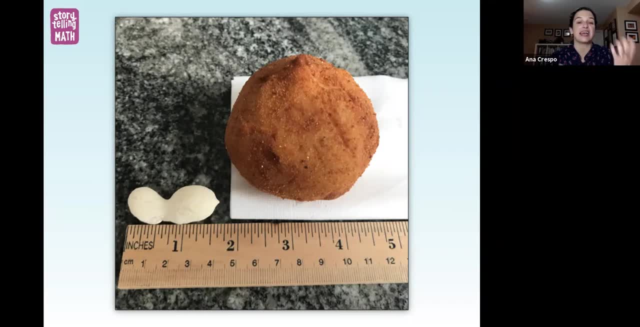 had to do was to substitute the lead and the cotton for food, And so, for the cotton, I picked biscoito de pavilho, the little white one there, which is a very, very airy snack, So it's very light, made with tapioca flour. So for comparison, think of Cheetos- It doesn't have that. 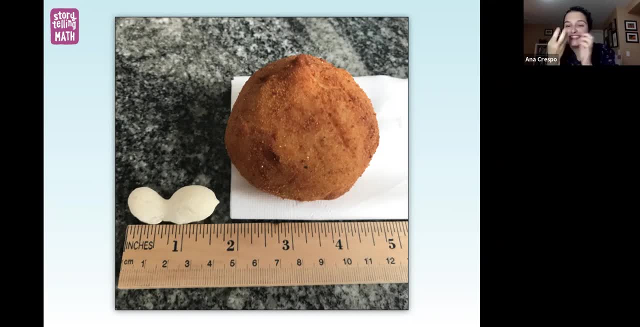 yellow thing that gets attached to your fingers and never comes out, And so it's like a very healthy Cheetos, I guess. And for the lead I picked coxinha de galinha because because it's made with this very heavy dough and it's filled with chicken and catupiry cheese. 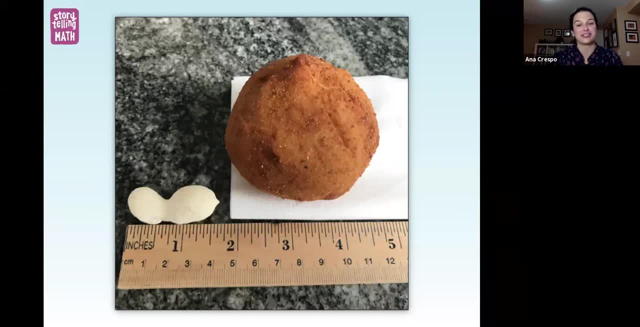 And so if you have a Brazilian bakery close by, you should certainly try those, And so anyway. so once those were picked, then it was a matter of figuring out the plot. Well, I have two younger siblings, very close in age, and we did fight a lot, really a lot. 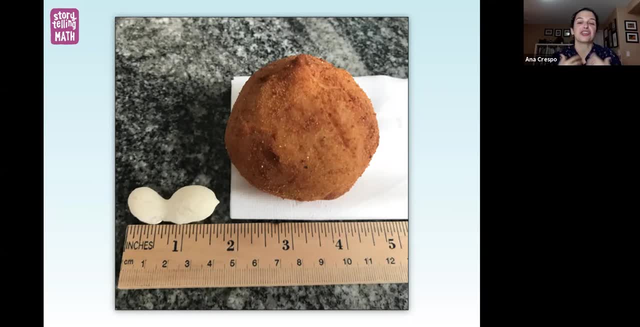 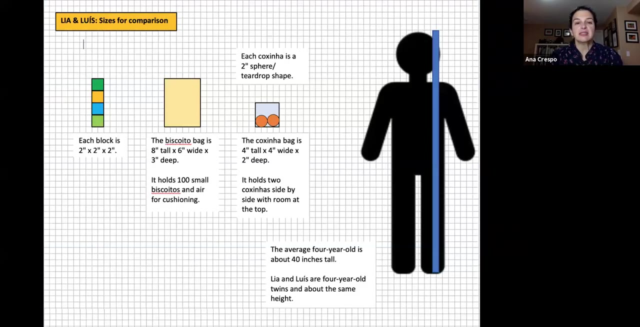 Right And sibling rivalry is such a universal theme that and so many people can relate to it. That's just, it was the natural way to go Now, if we can go to the next slide. So this book is only about 300 words long. 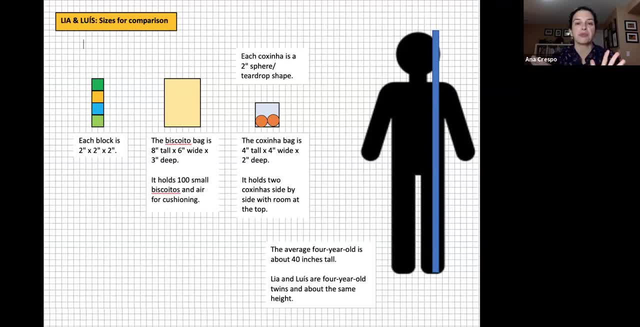 Right, I don't know the exact number of words, but it's around 300 words, And so often people are very surprised. When I mentioned all the back and forth conversations that Alyssa Marlene and I had, So in the image before this one, you saw that there was a ruler. 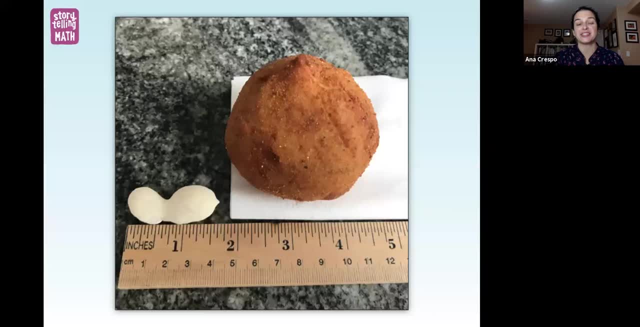 Well, I drove to the nearest Brazilian bakery, which is an hour away from where I live, And I bought some coxinha de galinha and some biscoito de povilho. And so I measured everything, weighed everything, aged everything too, which was the best part. 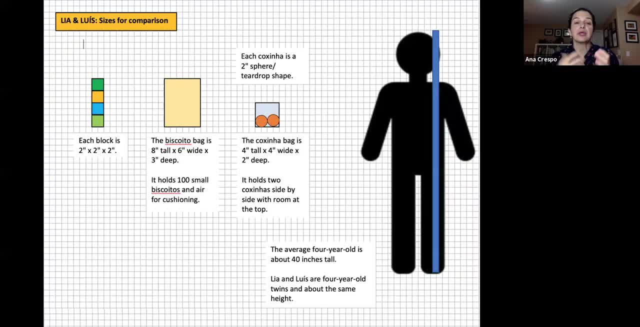 But eventually, what we had was that we knew that the coxinha de galinha weighed 75 grams, We knew that the bag of biscoito de povilho weighed 100 grams, And so we knew. spoiler alert, because I'm going to ruin the end of the book. 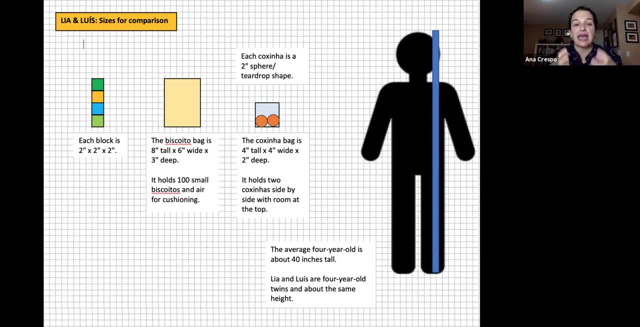 But we knew that for both kids to have the exact same weight of snacks, Leo would need to share about a third of the coxinha with Luis And, as you can see in the image right now, it didn't stop there, right. 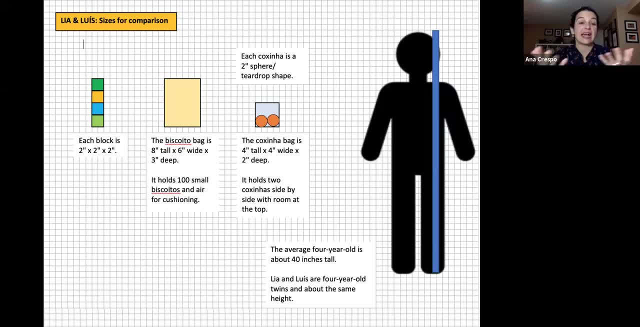 Marlene developed this guide, I guess with the details like the sizes of the blocks that are featured in the book, the size of the bag, how many biscuits are in the bag, all this detail to develop this book made the book extremely interesting. 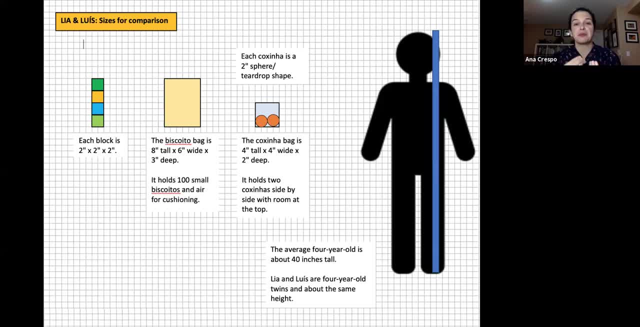 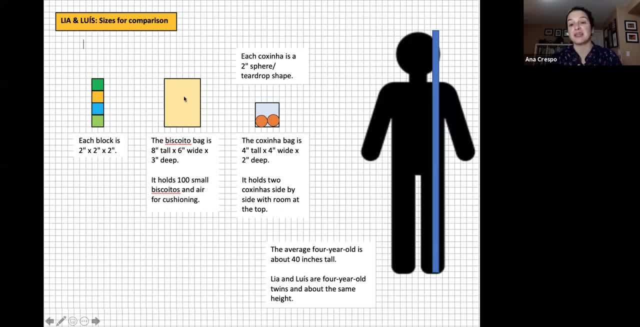 It's a very authentic, culturally, but also mathematically possible, which is something that I wanted it to be. I wanted it to be mathematically possible, So, anyway. so that's how Leo and Luis came about, And I think we do have a few slides with the first few spreads. 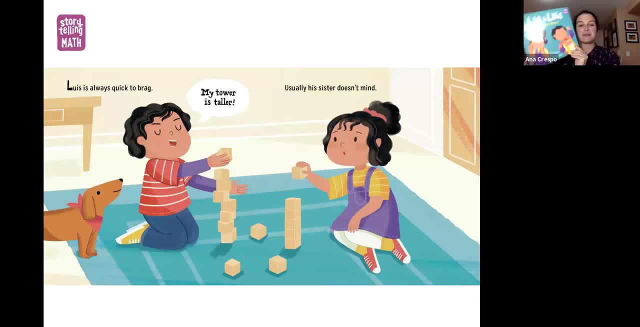 So this is the cover, one more time for you to remember, And I'm going to read it from the screen, Alyssa. So here we go. So this is Lee and Louise, Who Has More written by me and illustrated by Giovanna Medeiros, who is also from Brazil and so helps the book be even more authentic. 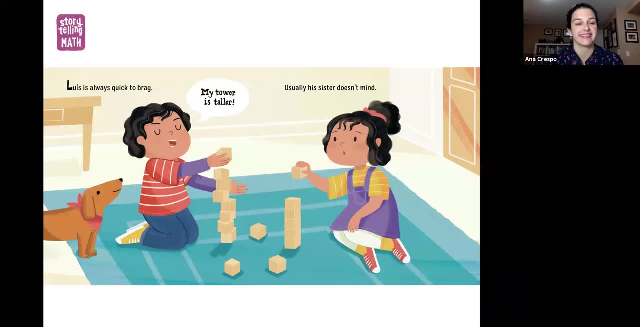 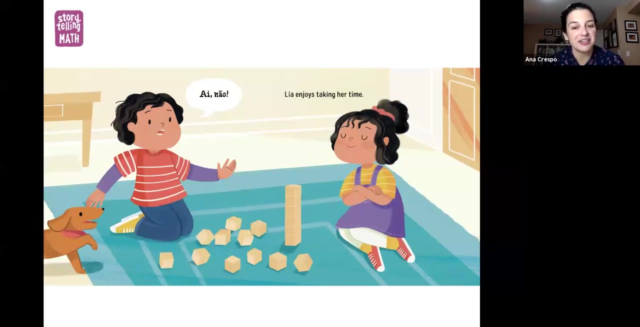 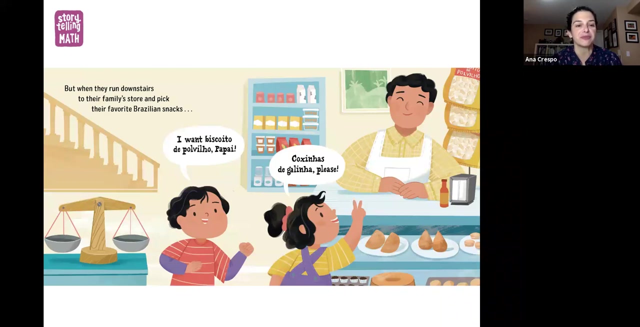 And it is published by Charles Bridge. So let's get started. Louise is always quick to brag. My tower is taller. Usually his sister doesn't mind. I know Leah enjoys taking her time, But when they run downstairs to their family's store and pick their favorite Brazilian snacks, 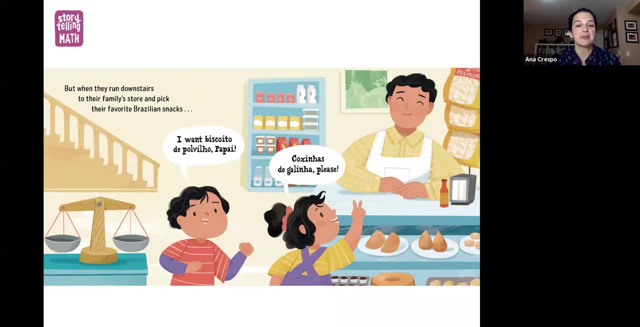 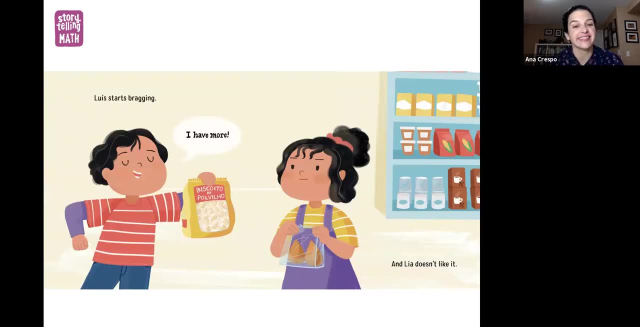 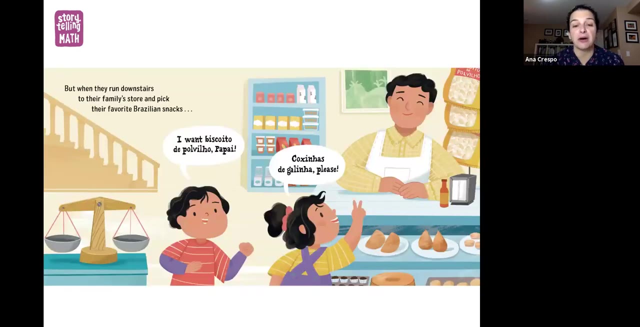 I want biscoito de povilho, papai coxinhas de galinha, please, Louise starts bragging. I have more and Leah doesn't like it, And so in the previous spread you'll see that, uh, I didn't write anything about it in the manuscript. of course this was all Giovanna, but you will see that. the image, the little snacks that you see close to Lia, the little black balls on the bottom, those are brigadeiro. they are Giovanna's favorite and very traditional Brazilian. 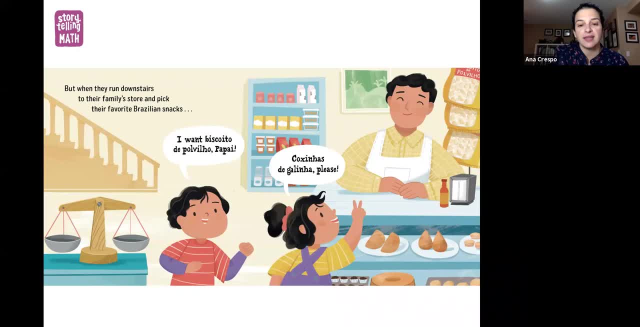 And there's like some milk pudding and some coxinha de galinha, some risole. all of that makes the book very authentic. A Brazilian kid who actually sees that picture will recognize all those snacks that are there. But I'll let Merlene talk a little bit about the math in the book. 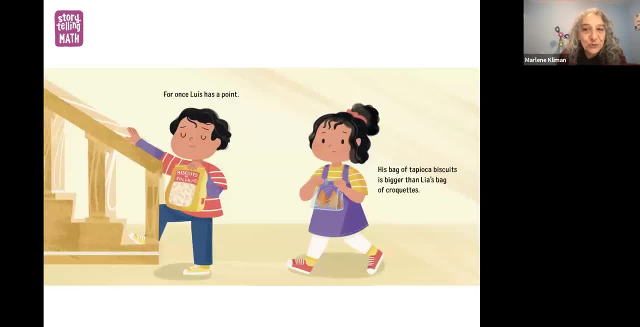 Lia and Luis throughout explore measurement exactly the way young children were invested by Really a hands-on visual comparing sizes, amounts and weights. We see their mathematical thinking in action throughout the book as they try to determine who has more And actually it kind of ups the tension. so it's very much connected. the math and the plot and the tension are related. You could even read through the book and barely even see that there's a lot of math in. 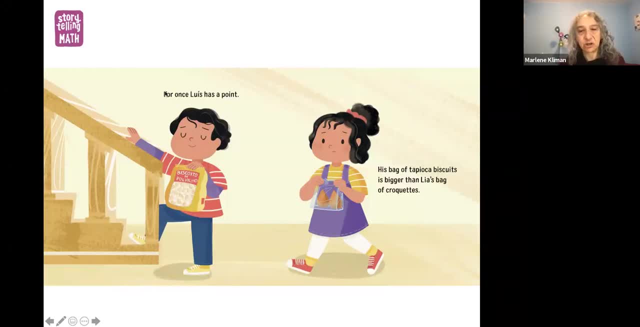 So first they do what the very youngest children reading this book would do is say: look at general size. So first they do what the very youngest children reading this book would do is say: look at general size. Which looks bigger? Well, Luis' package is quite big. Next slide, please. 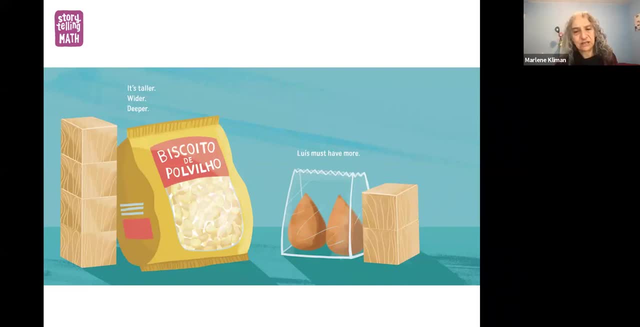 So as children move through the preschool and pre-K years into elementary school, they start noticing and comparing along three dimensions: length, width and height, And of course this is relevant for older kids. It's taller, it's wider, it's deeper. So they start unpacking big. to just what does it mean to be big or bigger? 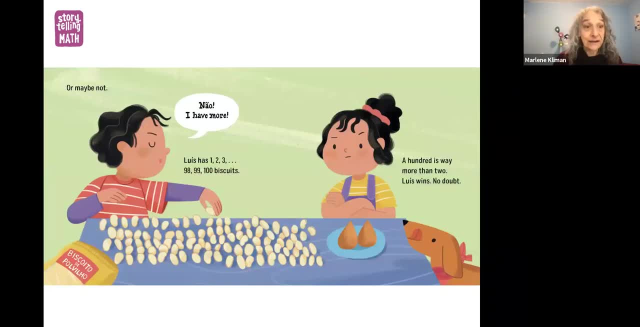 Next slide. Another way they try comparing is by amount: 100 little biscuits in the bag versus just two croquettes. Now, even if the readers are way too young to count 100 objects, they know that there are a lot more biscuits. 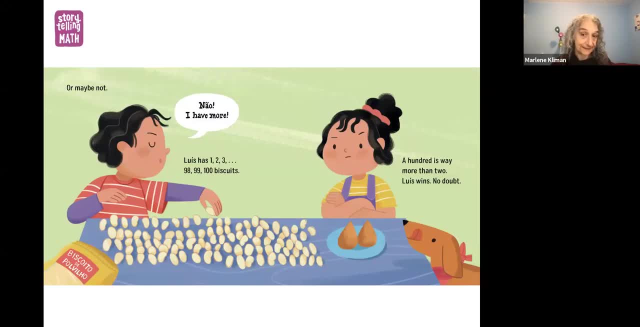 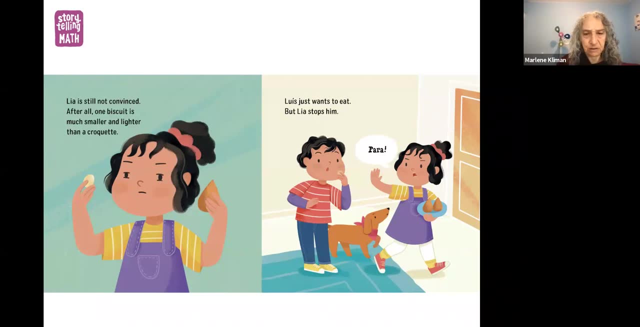 So who has more? It certainly looks like Luis does Next slide, please. But then Leah thinks about weight. She holds them up, Next slide please. And then Biscuit. she notices it's much smaller and lighter than a croquette. 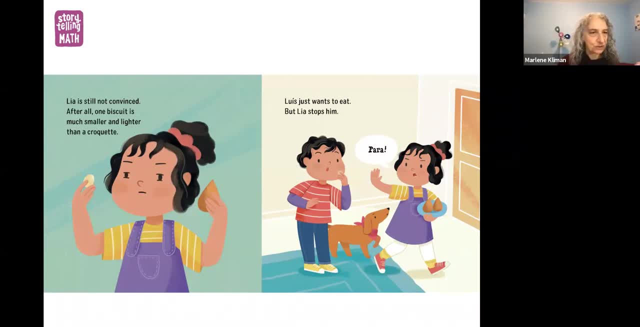 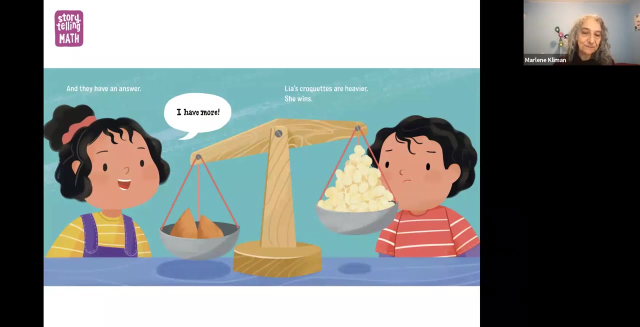 So she's actually starting to make sense of density. We don't use that word because this is an engaging story. It's not a lesson, But density is key here, and it's a topic that spans math and science. Next slide: So finally, they decide to compare by weighing. The balance scale gives children a visual representation of comparing weight. 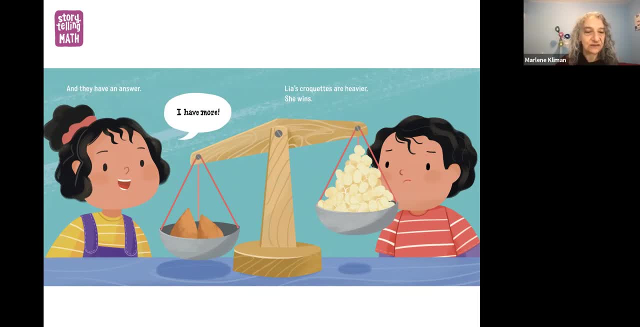 Long before they can meaningfully compare, say, pounds and ounces, or calculate density. All the comparisons that they make are very age-appropriate. They reflect the way young children really think about who has more, And it's probably something that's very familiar to readers. They may not have thought about it as math but, as with Circlesphere, it gets these math ideas out on the page. 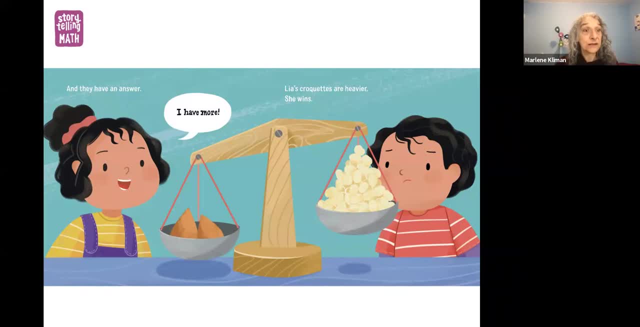 so that readers can naturally reflect on and talk about different ways to compare. Next slide, please. Next slide, please. One take is to measure and compare And see before we go on to the activity. Anna, were you going to talk a little bit about some additional thinking about ways that could compare that came up in one of your sessions? 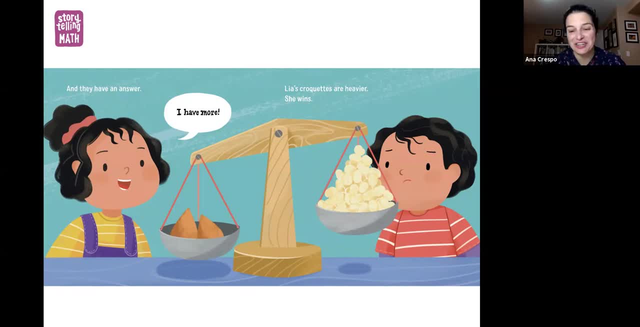 Yes. So Marlene was excited when she heard the experience that I had during a virtual visit at a school. So I read Lee and Louise and these were first graders And this one boy raised his hand. And of course, with children, you never know. 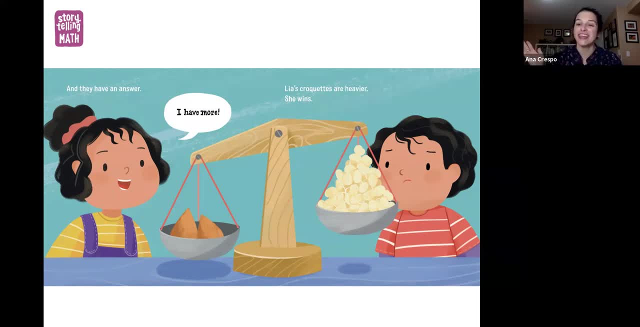 what it's gonna come out right. a lot of times they ask: do you like cake or what is your favorite color or something, and you don't know if you're connecting with them. but this one boy raised his hand and he said: well, if they put 50 biscuits on one side and 50 biscuits on the other in one? 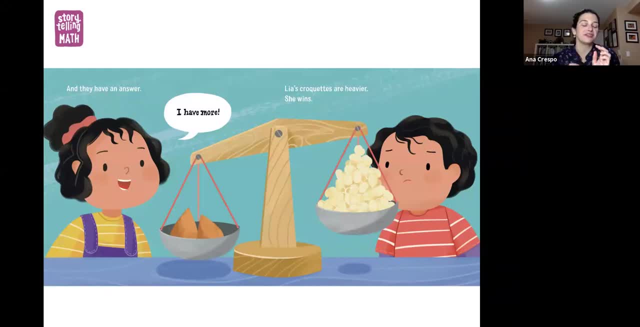 and I don't remember- I think it was croquette the word he used in- one croquette on one side and one croquette on the other. it would be the same too, and I think that's the kind of thinking that Merlino is really hoping that the kids would come out of it, and so she was excited to hear. 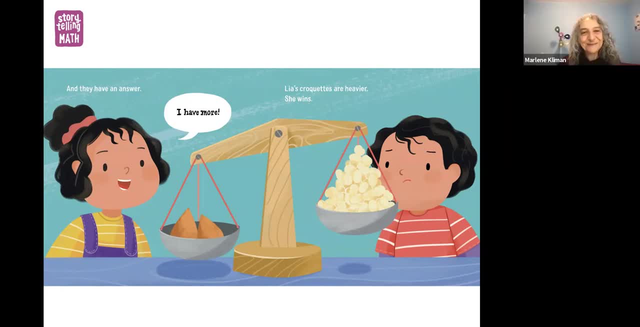 that experience and you don't know if the kid may have been thinking about it as math or may have been thinking is: I have a sibling and this is what I would do to make it fair, because I've been in that situation before, so it just gets them reflecting and talking. 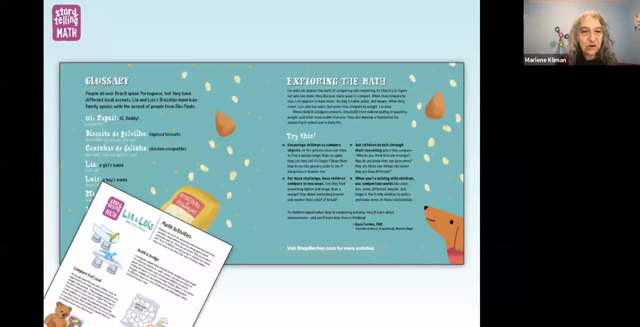 so next slide, please. so here you see information about the math and some activity ideas that allow for further exploring the math, both at the back of the book and they're. they're available as free downloads, and we also have a Brazilian- Portuguese glossary, and Anna is now going to show you an. 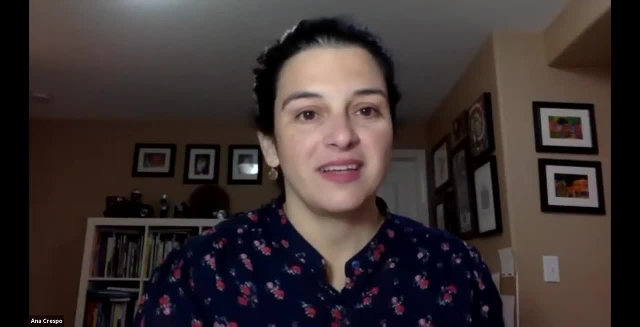 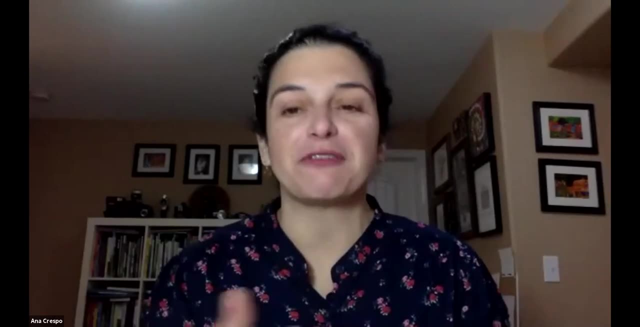 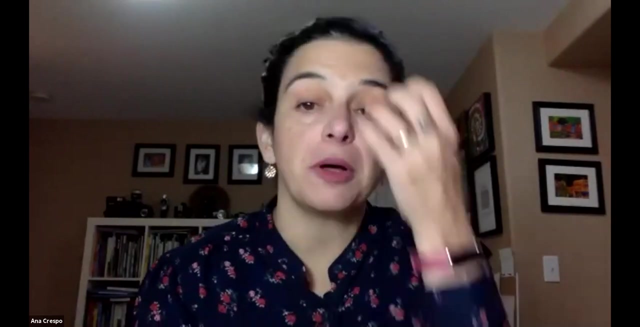 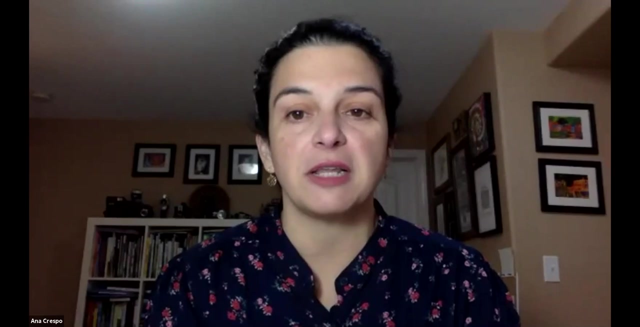 activity. okay, so I'm very big on this screen right now. okay, so there are many different activities, of course, that you can do with this and, like Marlene said, Charles Bridge have them available, has them available on the website if you want to download them in different languages. in the case of Lee and Louise, it's. 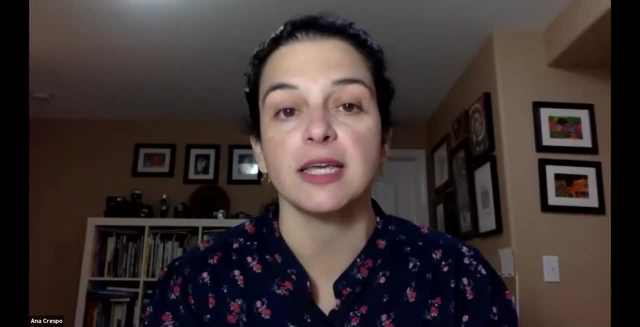 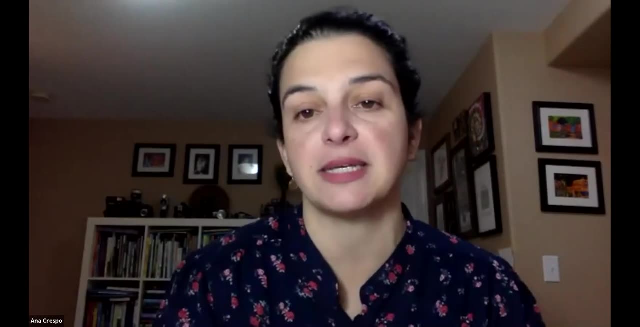 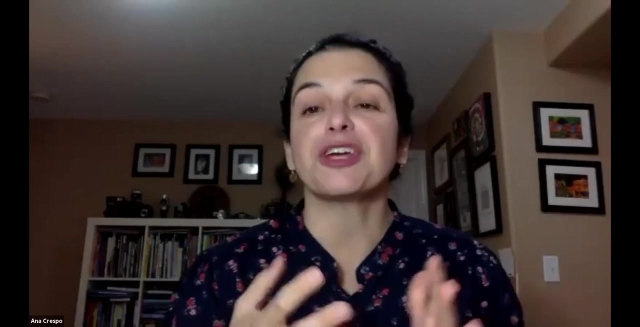 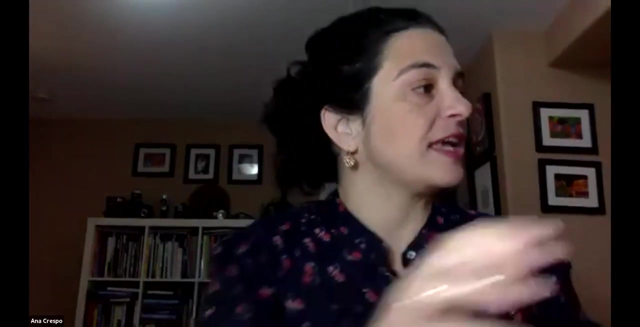 available also in Brazilian Portuguese, but other books like Luna- I forgot the title, but Luna's book is available in Chinese as well, as far as I understand. so there are many, many options there on the website. you should certainly visit it, but for this activity you're going to need a beach ball, a soccer ball and a baseball and you can start. here's the. 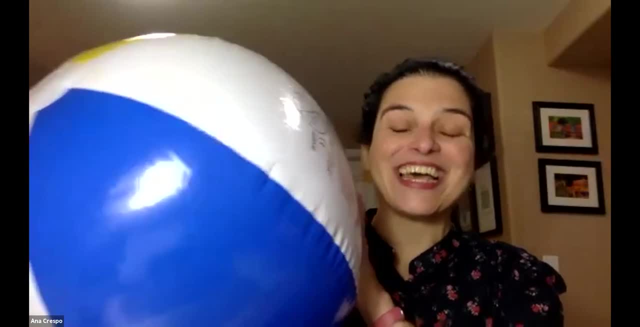 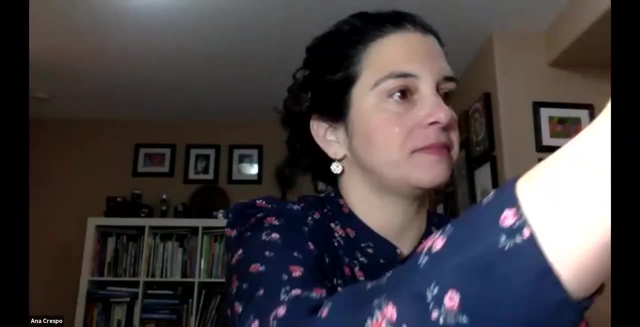 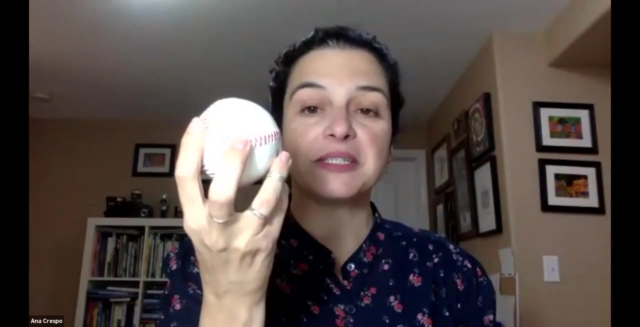 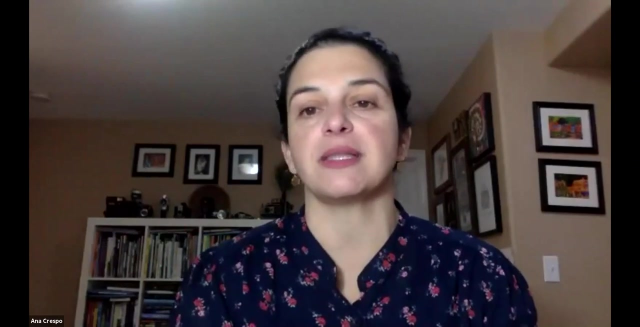 beach ball that took me almost an hour to inflate, but you can start in here. I just want to show you what I have here, so the soccer ball, and I cannot put them all on the screen together, so in the baseball right, and so you can um start by asking the students to describe each one of the balls and they might say like one is. 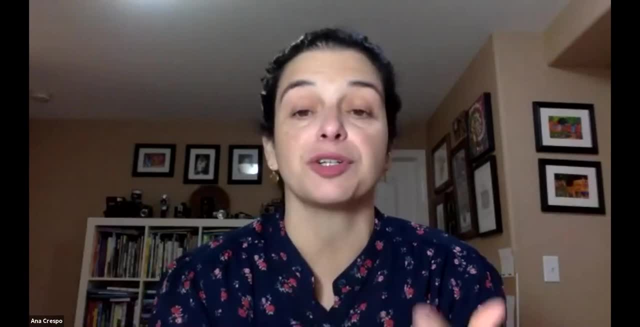 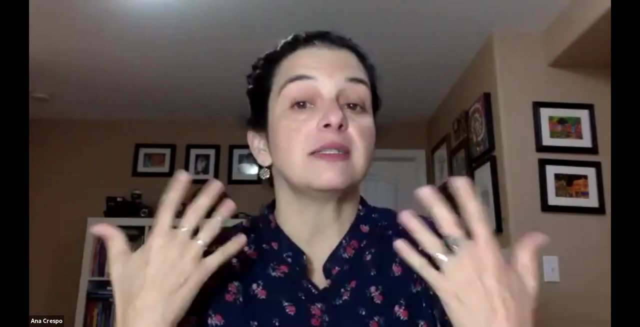 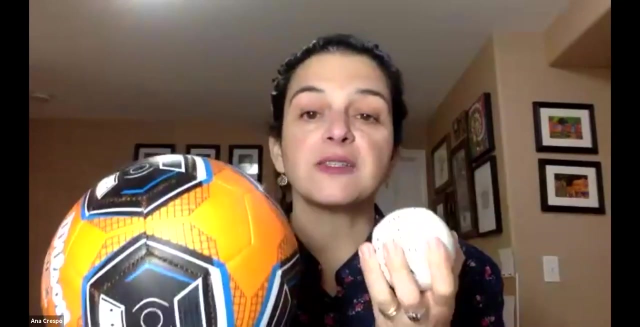 colorful, the other is orange. but hopefully at some point they're going to mention sizes as well, and if they don't, you can always prompt to them and ask which ball is the biggest, which one is the smallest? is the soccer ball bigger than the baseball? is the baseball is smaller than the? 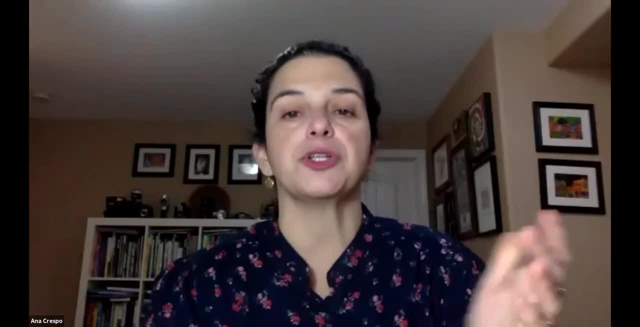 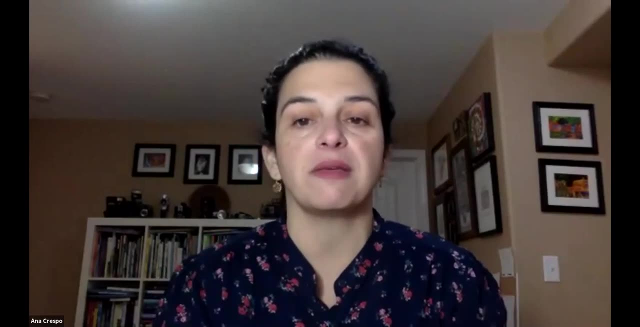 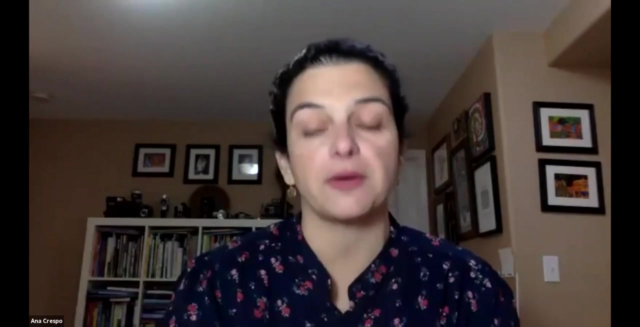 And so it goes, And notice that when you're doing that, you're not only encouraging the mathematical thinking by comparison itself, but you're also helping them develop their comparative and superlative knowledge, making this really an interdisciplinary activity that makes us both language and math. 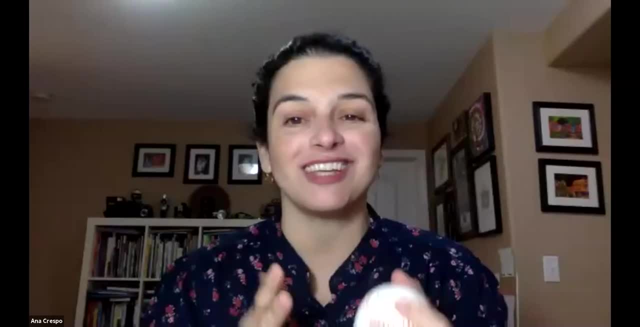 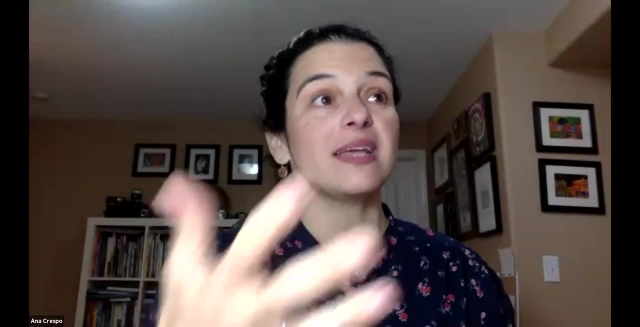 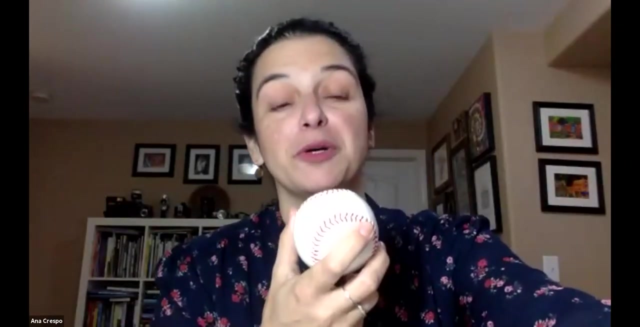 Then ask them: which ball do you think is the heaviest? right? Because that's like, if you think about the question that prompted Lee and Louise, the beach ball would be the cotton and the baseball would be the ledge. One is much, much bigger than the other, but the beach ball is lighter. 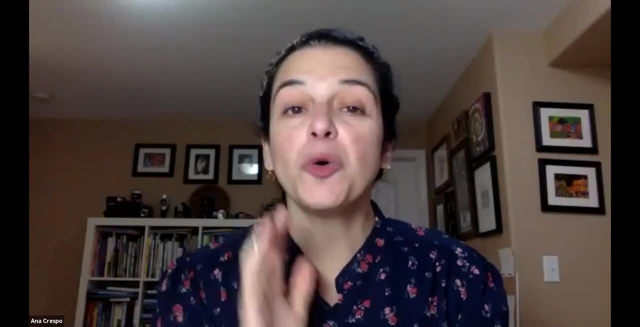 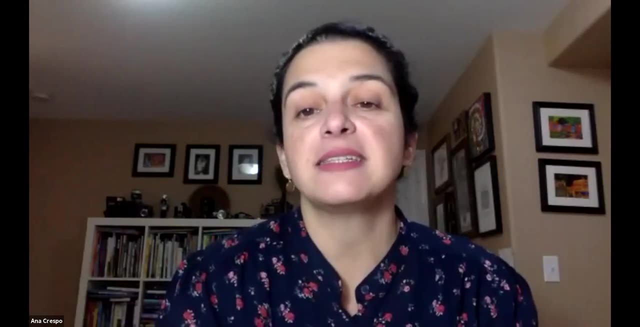 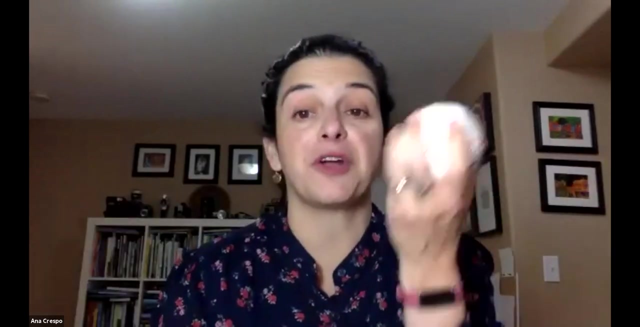 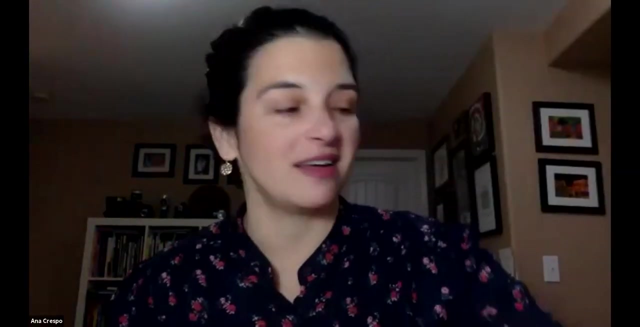 So, anyway, have them guess the answer, and only them then, And allow them to hold the balls and actually feel which one is heavier and which one is lighter, So can they put the balls in order from the lightest to the heaviest which just fell on the ground. so I'm not going to get it- or even like from the smallest to the biggest. 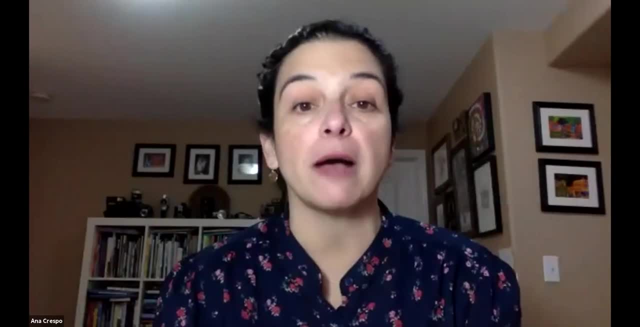 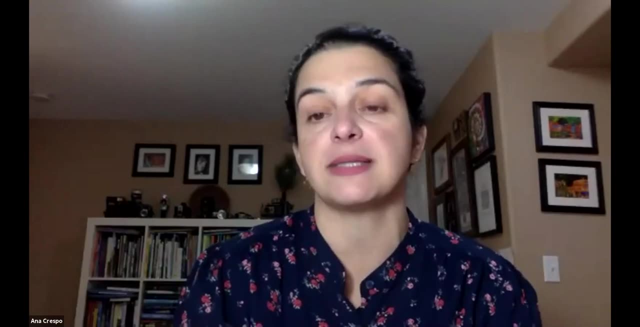 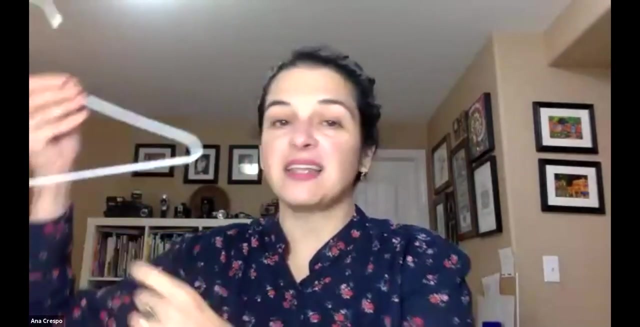 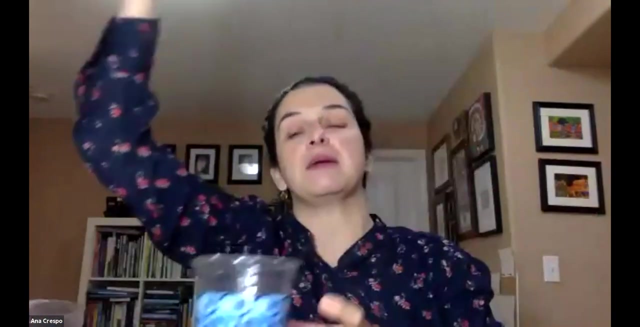 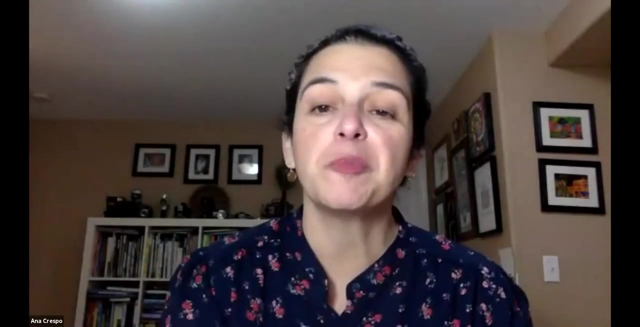 So there's a lot that you can do with this, And these are such simple Objects. you can use them inside the classroom, where you can take them outside and have them kick the balls and experience them in a different, different way. I also encourage you to make a balanced scale with. you just need a little hanger, like some string and some disposable cups, and the kids can start weighing everything around, from Lego pieces to 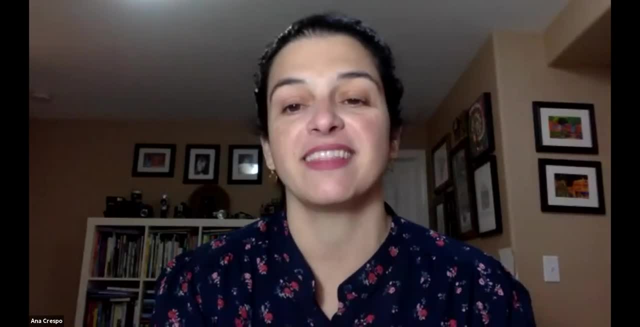 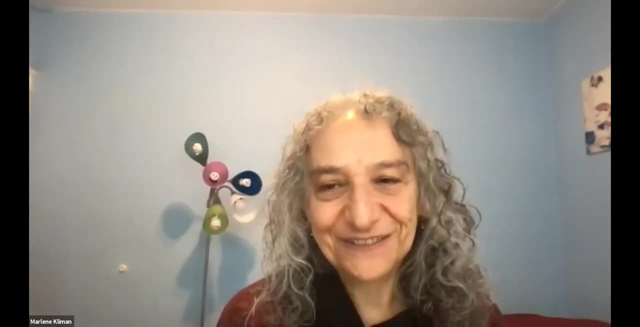 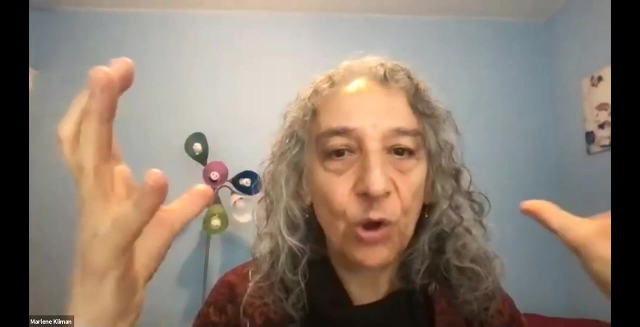 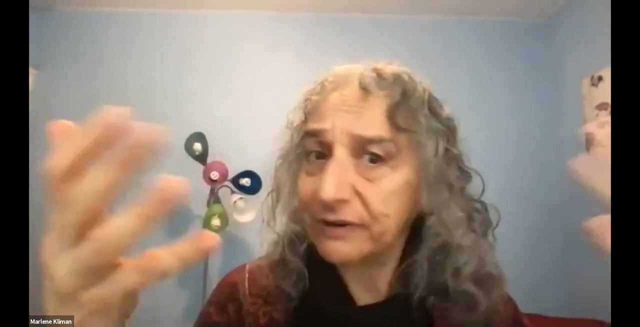 I also encourage you to make a balanced scale with. you just need a little hanger like some string and some disposable cups, and the kids can start weighing everything around, from Lego pieces to при des. Two ways to get that flip. 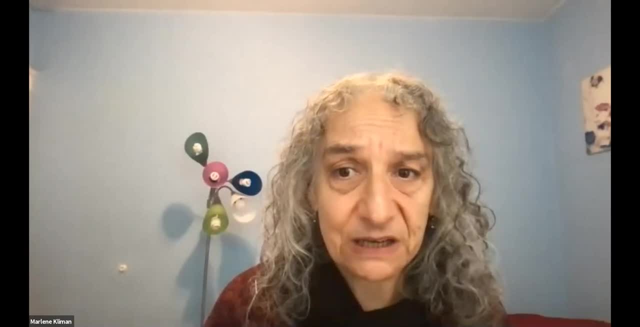 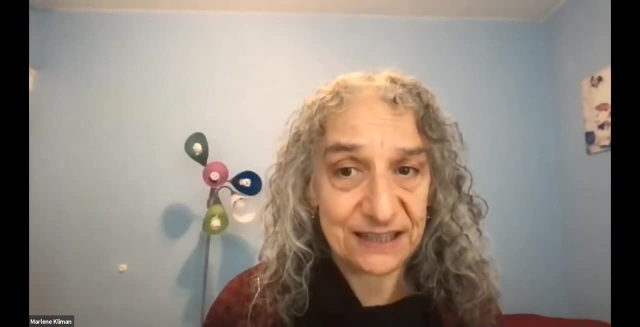 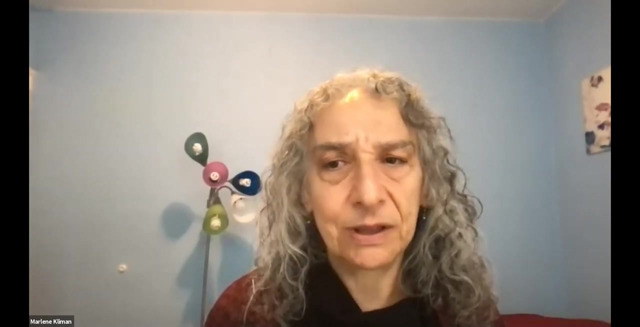 était that flip. It's not because of the- you know elementary school project based on it making the hangers or talking about which weighs the most, because it kind of broaches the concept of density. Kids start having to do density calculations and they meet density in science and math in elementary school. 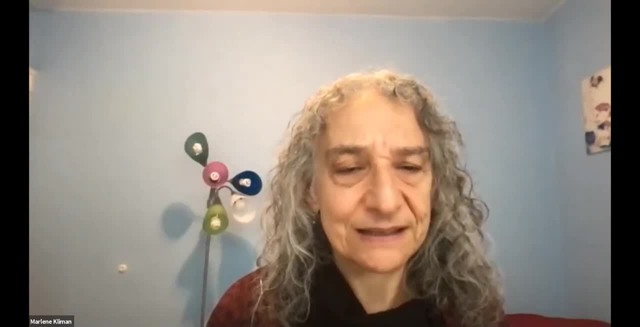 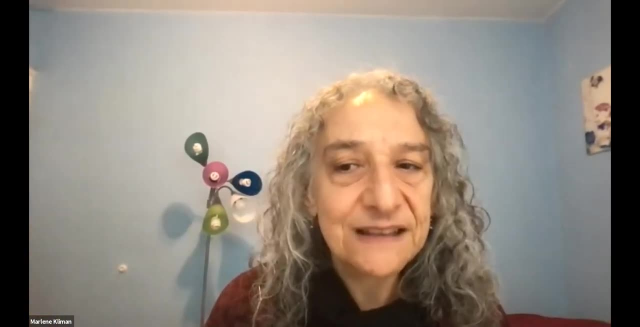 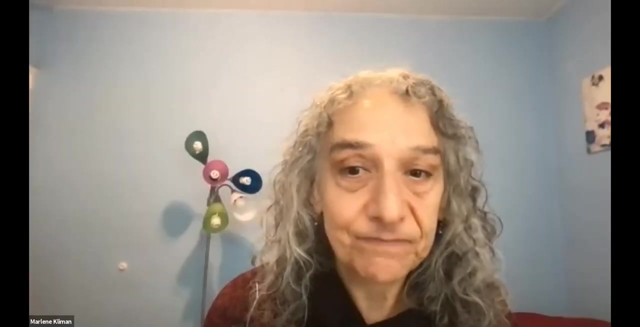 but often they have no real sense of what that means. And if you imagine you know a baseball versus a beach ball, well, that's density right there. So activities like this give all ages a chance to build that underlying understanding. Thank you, 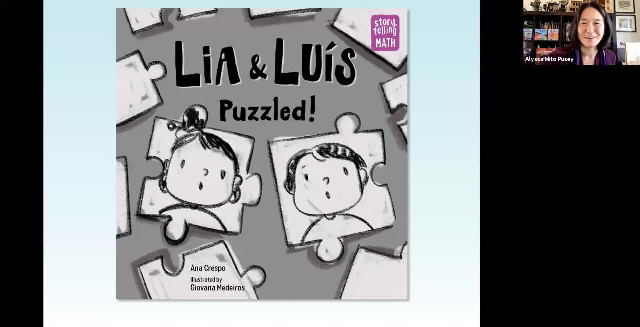 Thank you, Anna, And now I am going to give you all a sneak peek at what Leah and Luis are up to next. So coming next fall is Leah and Luis Puzzled. Grandma sends the twins a gift, a puzzle, and can detectives Leah and Luis put it together to read the secret message? 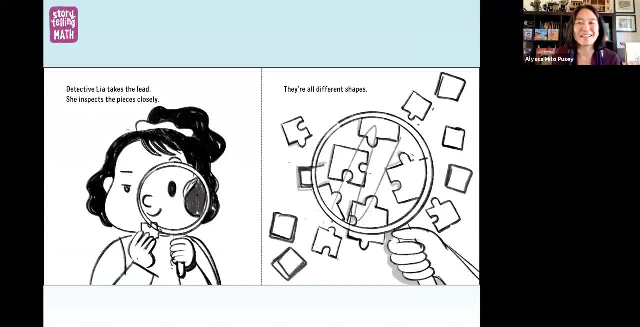 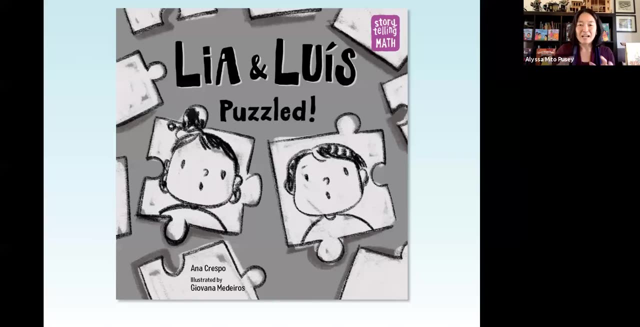 And then we see. We see Detective Leah, who is just so cute And, spoiler alert- the message says that Grandma is coming to visit, So puzzles are a fantastic way for kids to develop their spatial skills. As they put the puzzle together, Leah and Luis are exploring shapes and rotation and logic, and 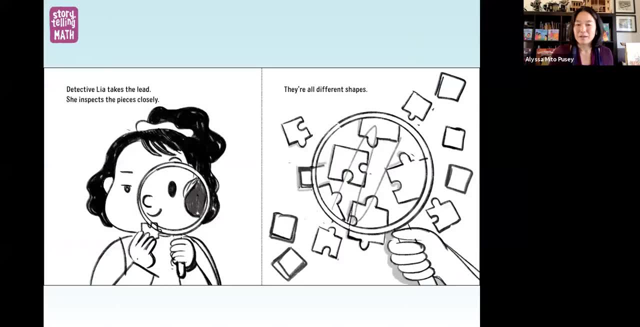 sorting, And right now Giovanna is developing the sketches and working with Anna and me and the art director to figure out what elements of Brazilian culture are going to be throughout the art. And that leads, And that leads us to our last conversation about the importance of diversity in children's math books. 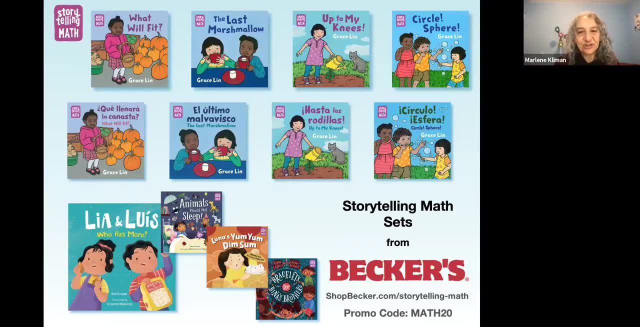 Okay, I think Next slide. yes, So all of these books show children of color as strong mathematical thinkers as well as fully realized characters. Young readers of color need to see themselves reflected in math picture books and all readers need to see children of color engaging in mathematical. 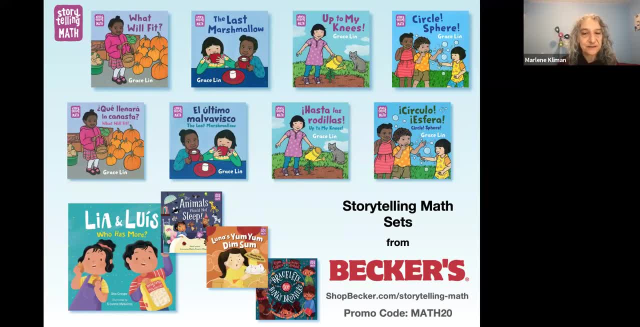 thinking. Research shows that stereotypes about who is a mathematician are not necessarily the ones that are the most important, And so we need to see children of color engage in mathematical thinking. Research shows that stereotypes about who is a mathematician are not necessarily the most. 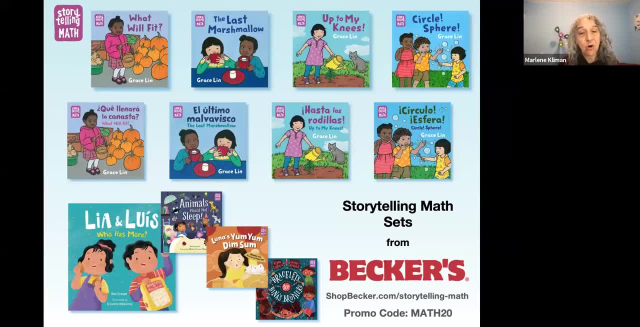 important, And so we need to see children of color engage in mathematical thinking. Research shows that stereotypes about who is a mathematician are not necessarily the most important, And so we need to see children of color engage in mathematical thinking. Research shows that ever 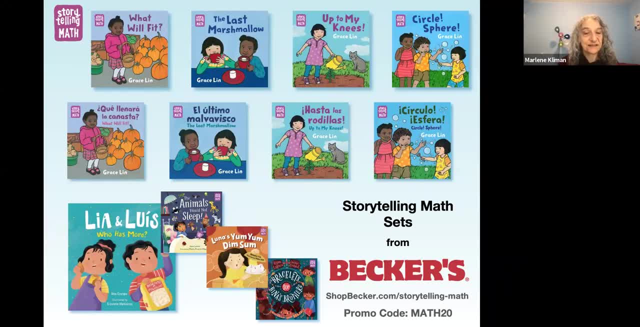 again, it is requesting the attention of their parents to hold a TI of sort. We need to feed the kids. we can think about based on the betterません and then change the way we think about things based on the best sense of blackness and's overall meaning, and that's why we're working. find. 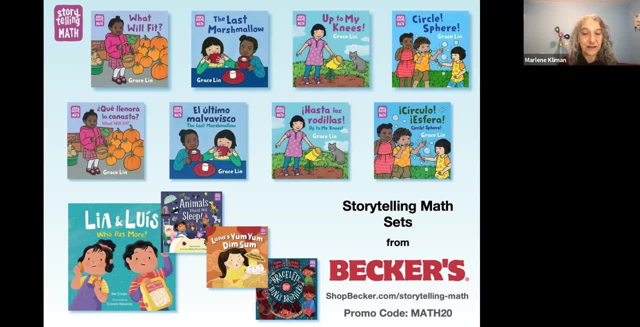 ways to dream about the future of order than just offices. We really need to so we can do any job in does well there, But also we need to see who is better and who isn't And who is not can generate a literally see children of color as strong mathematical thinkers. 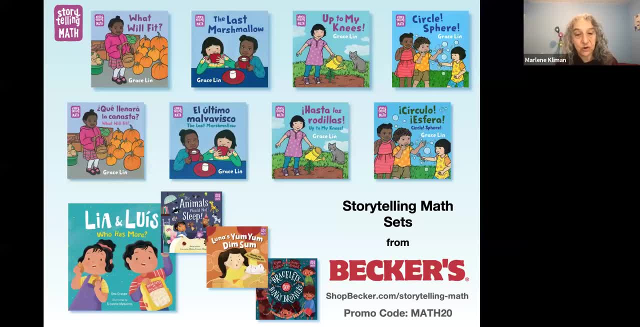 Again, research tells us that children who start school with strong early math skills are more likely to succeed in all school subjects, including in reading. We want all children to have an opportunity to experience that success. So others want to join in and talk about it or talk about the other books. 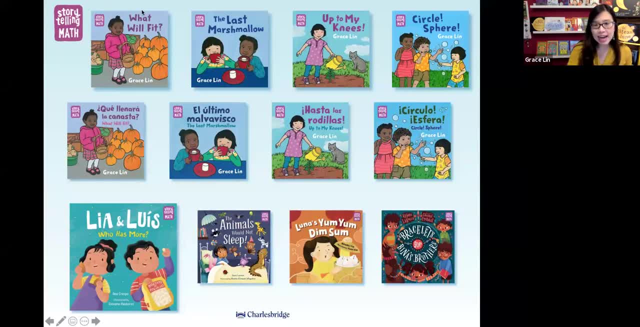 I thought I would. this isn't exactly about math, but when you were talking about modeling, I thought that was such a really important thing like modeling, how kids can see themselves, And we talk about this a lot when we talk about diversity too. you know that kids 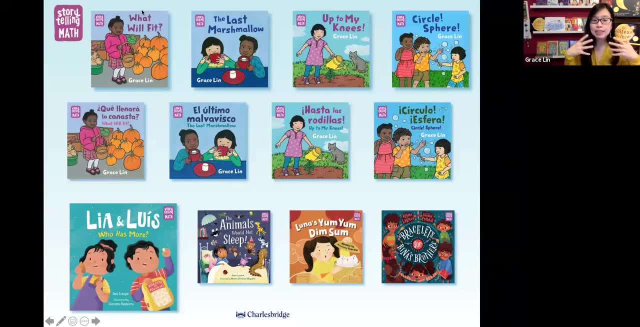 need to be able to see themselves in a book. They need to be able to see themselves as a main character of a book because by seeing themselves as a main character, they can see themselves as the hero in their own story. It empowers them, right. 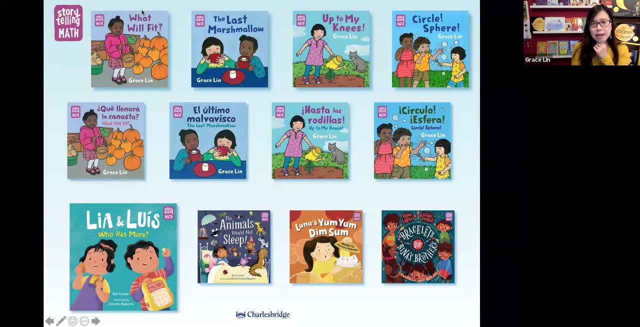 One of the things. this is one of the things that has happened in my experience. So, as you can see, I've been publishing books for quite a long time And I've been visiting schools for quite a long time, And I remember at one school- this was probably fairly early in my career, I would say- 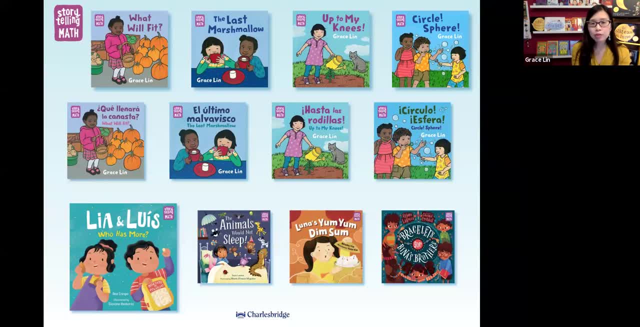 This is probably 15 years ago. I remember the principal came to me and he said: oh, I am so glad that you came to our school. We're making such an effort to get more diverse models for our kids. And I said: oh, that's so wonderful. 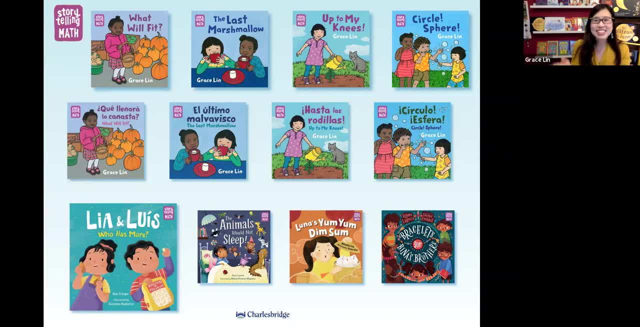 Why I'm just so curious, Like what? Because, remember, this is like 15 years ago, before diversity, before like we need diverse books, before all these things, before people were really aware of it. And so to me I was very curious. 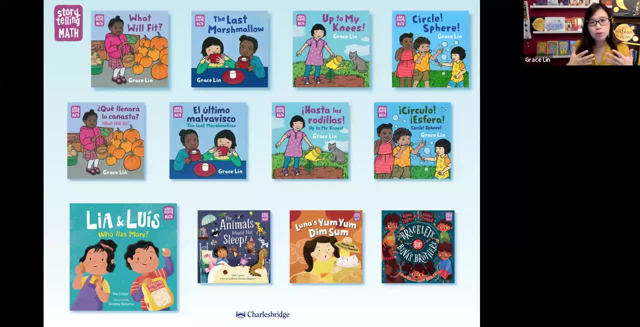 Like: I'm so glad that you are thinking about this, But what brought it on? He's like: well, the truth is, a couple months ago I was hanging out after school And there was like this after school program And there's a mother and a son. 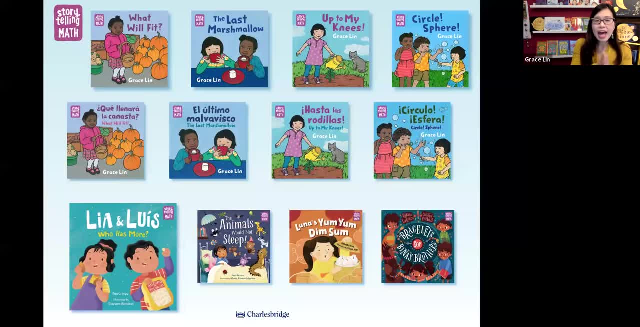 They were both black. They were sitting in the gym, I think they were waiting for something. And the mother was saying to the son: what do you want to be when you grow up? And he's like: I don't know. And she said, well, how about a fireman? 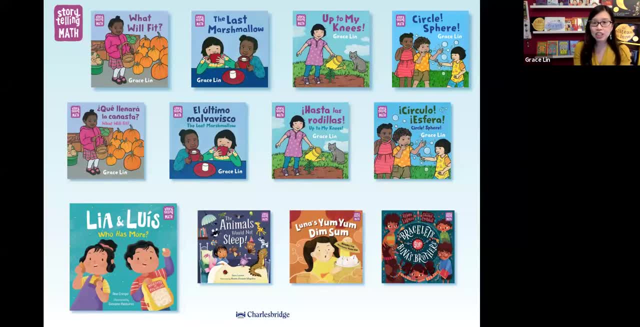 And he's like: I don't know. And then she's like: well, how about a teacher? And the boy said: I can't be a teacher. All teachers are white. And the principal said: that broke his heart so much. 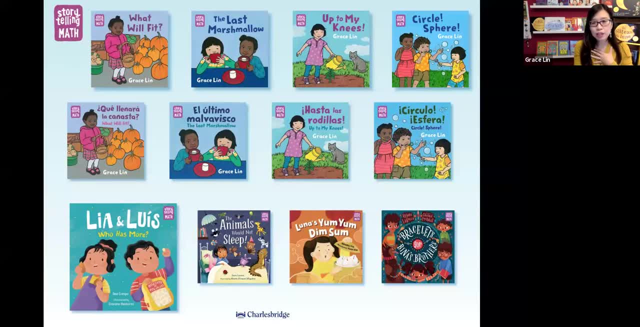 But then he looked at his staff and he realized that is what this boy was seeing: All the teachers were white. And so by seeing that he, this boy, felt like that was not something for him, And so by bringing authors in of color by and remember, like I said, this is like 15 years ago. 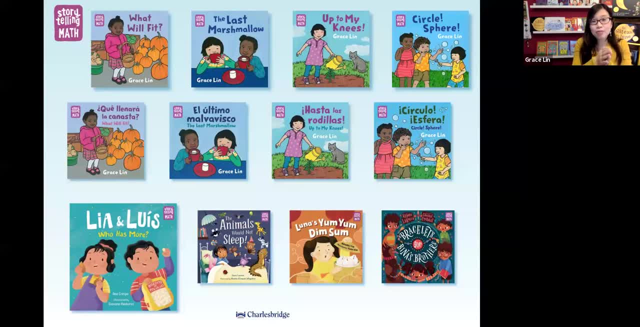 when there were diverse books was really really just not a thing, And so and the bookshelves were didn't show anyone that looked like the student either, or very few, Or the ones that did were about civil rights and slavery. 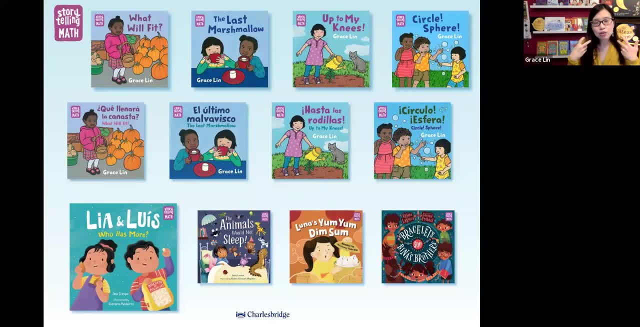 You know like those are things that kids start to ingest And there's nothing wrong with those books. But if those are the only books, they start thinking that those are the limits that they have, And this series is such a wonderful way to show kids that they are unlikeable. 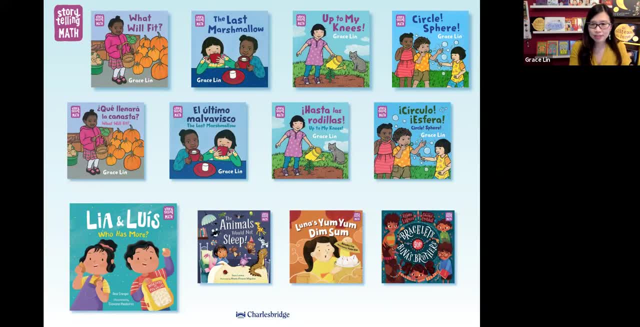 That they are not limited. That's great. So you see there's a few other books. they all are that that Becker's has in the series. they're all have strong math, a powerfully emotionally resonant story and diversity. They show kids that they deserve to be in books. they don't just deserve to be in history books, but kids of color deserve to be starring in their own stories. 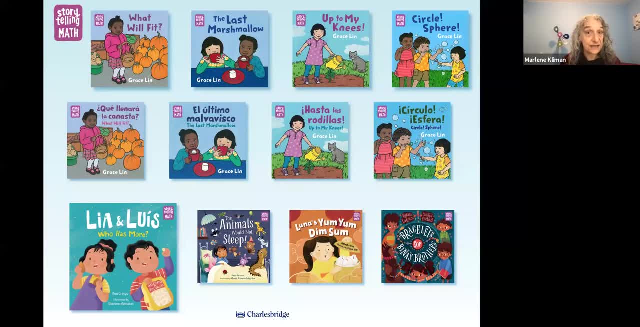 So in bracelets for being as brothers, That one centers on the Indian House, That one centers on the Indian House, And it's a little girl trying to prove herself to her big brothers. and the math of patterns- The animals could not sleep- blends the math of sorting and caring. it's a real empathy story with classifying and logic. and in Luna's yum yum dim sum, Luna and her two brothers puzzle over how the three of them can share five buns fairly. 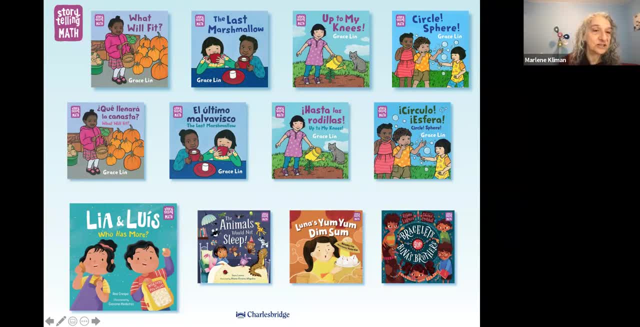 They grapple with division and fractions without actually using symbols or equations. They grapple with division and fractions without actually using symbols or equations, So they do it in a very age appropriate way. So they do it in a very age appropriate way. All the books have math information at the back, activities at the back and additional free download activities. 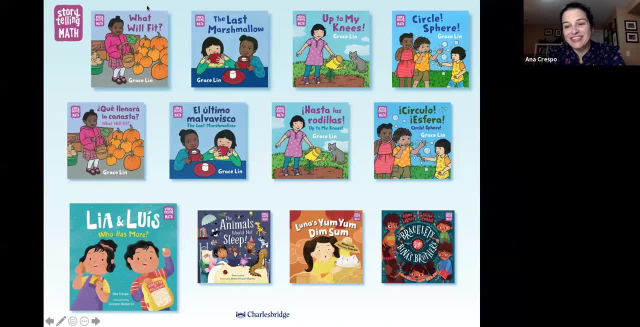 And one thing that I started saying. but then I noticed how is muted. So no matter how long it's been right, you always start talking and it's still muted, But anyway. but I had a similar experience to graces, But anyway, but I had a similar experience to graces. 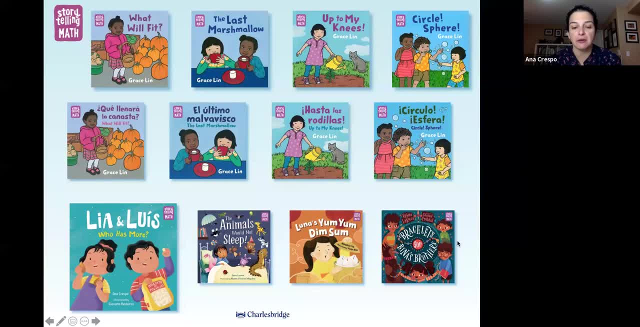 But anyway. but I had a similar experience to graces years ago when my first book came out and I went to a school and I had to introduce myself to the lady at the front, at the front desk so that she could let me in, and this one kid was coming in at 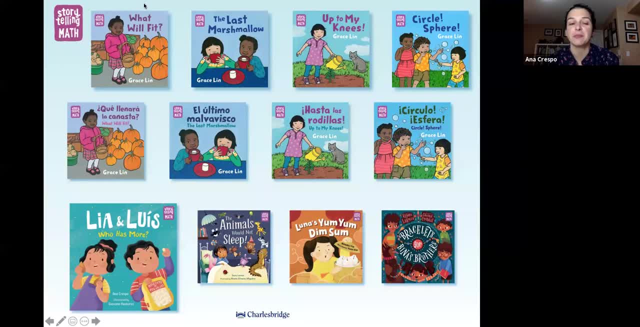 the same time and she was Latina. and she, when the lady asked me, so who are you? and I said, oh, I'm Anna Crespo, I am the author. and the little girl looked at me and she said you were the author. and I was, yes, I am the author, and and with me especially, I think, what happens as a mom too, and 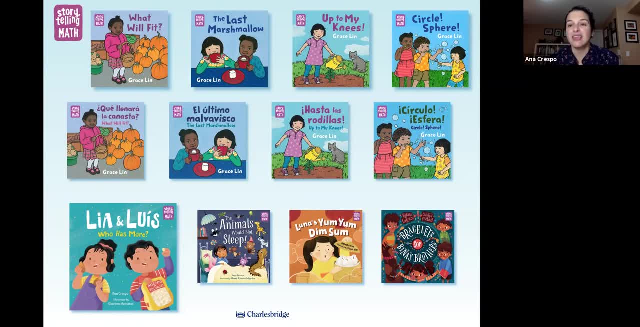 also as the as an author, is the accent. the accent makes a difference, so a lot of times people make assumptions based on the accent, right? so maybe English is not your first language- which is not mine- and of course you're going to have an accent when you're speaking a second language. 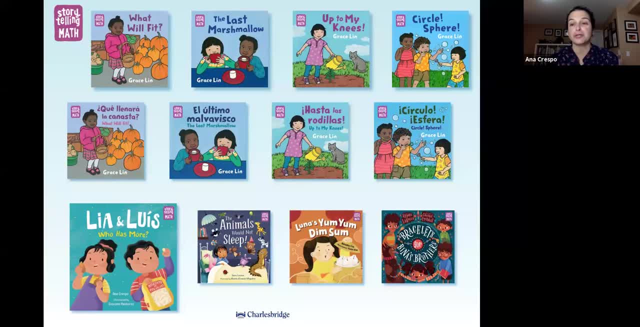 but that doesn't mean, for example, that you don't know math or that you don't know science, right, but a lot of times there are expectations that come with with the simple accent. you hear an accent and you assume that this person knows less than you, or or that this person is not capable of understanding something. 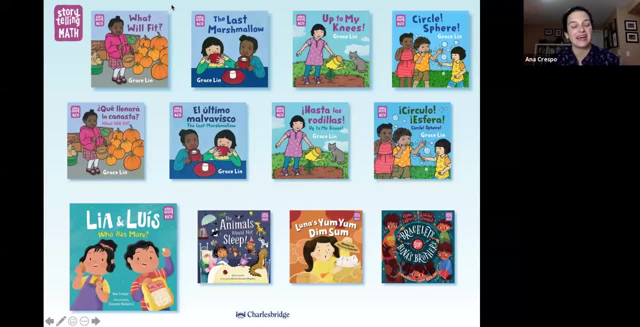 and so anyway. so, yeah, yeah, I think it's. it's very important for the kids to be able to see themselves in the world and to be able to see themselves in the world and to be able to see books, but also to be able to see diverse authors and diverse illustrators being authors and talking. 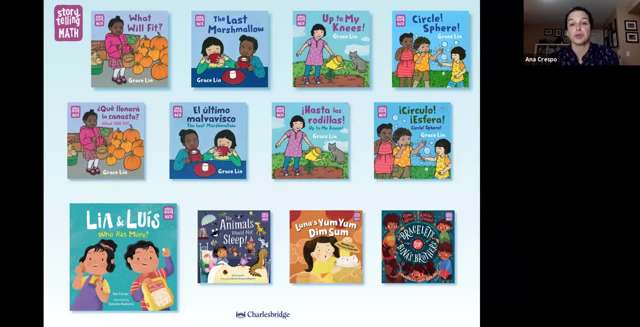 to people and being, you know, experts on something. that's also all very important as well. so I'm glad Grace shared that story. that is a very good story. um, I see that somebody um says in the in the question and answer: someone asked why board books and uh, uh, Alyssa. 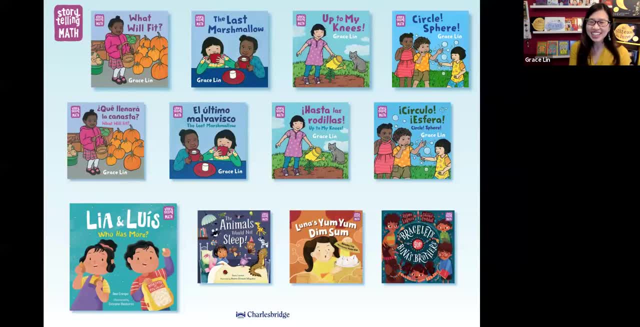 do you want to start the answer for that, or do you want me to? do you want me to try? well, I should have said from the very beginning that, um, the board books are intended for ages zero through two, and then the picture books are for ages three through six. and uh, we were. 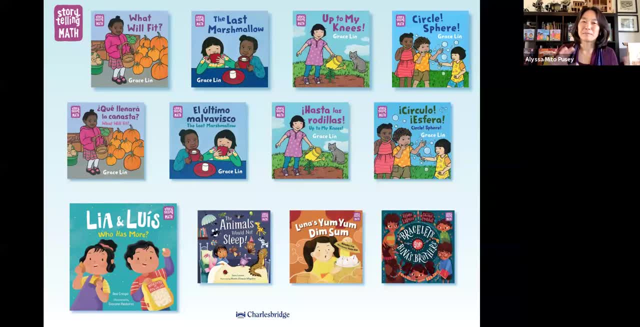 Marlene was very, very thoughtful and careful about developing the math for the right age group, and so she she was always saying: you know, kids of this age know they? they know this about spacial sense and then, as they grow older and learn more, they know this. and um, Marlene, did you want to talk? 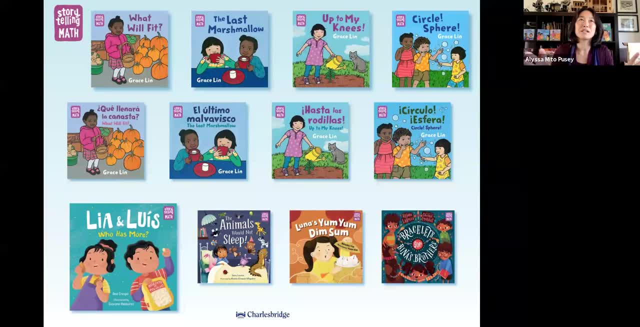 a little bit about the specifics, so so the, the series is very much age appropriate. just to let you know, Marlene, how. how the question was posed was- I'm not sure if you're looking at it is: why did you choose board books? how young will a child understand them? 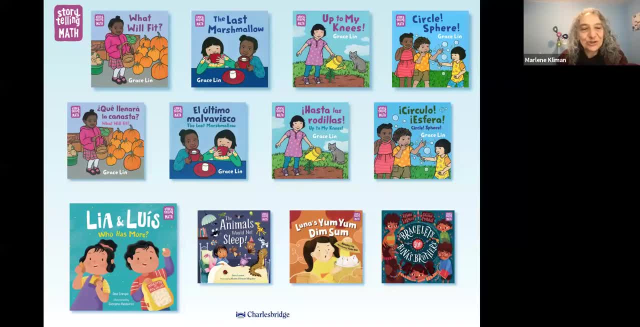 just to let you know, Marlene, how how the question was posed was- I'm not sure if you're looking at it- is: why did you choose board books? how young will a child understand them? Okay, I would you know. children learn math from birth. They start classifying things They know. 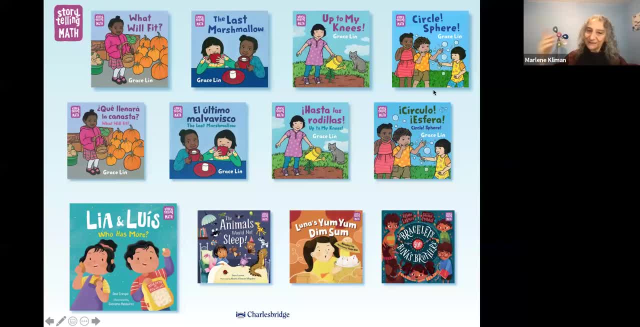 which you know who's my parents and who isn't my parents. Well, that grows, that grows. They know dark and light, They start discriminating colors and objects, And what we're doing is taking that early math. Yes, there's a lot that children learn naturally and organically. 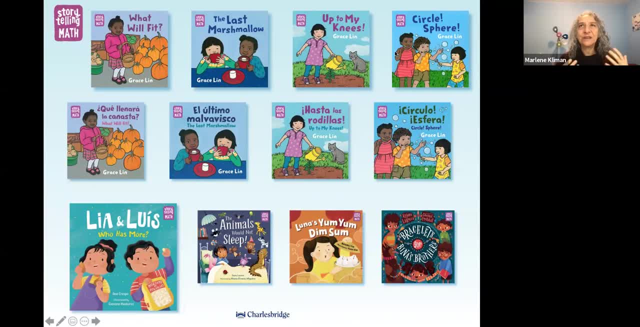 but we're giving you a chance to talk about it. We're showing it to you on the page, sort of formalizing it. As Grace said, it's all around us, but we're choosing a few elements to put a spotlight on so that children and their caregivers see it on the page, can then start. 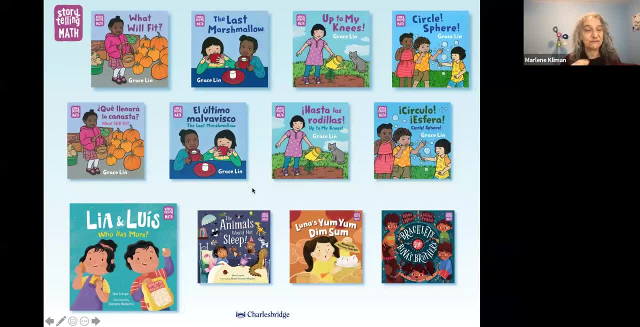 looking in their everyday lives for it. That's why we conscientiously didn't write fantasy, didn't write you know history. We wanted it to reflect what's in the world of a child in the United States right now, or a child in the United States. 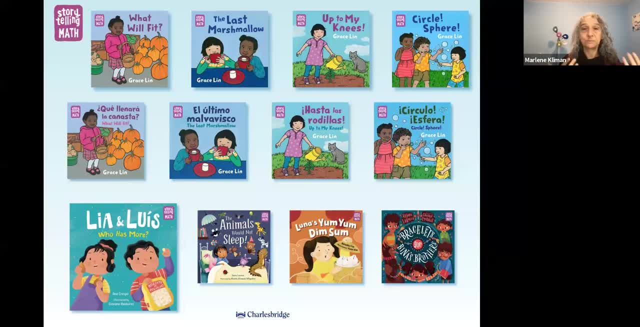 who may well come from another country or who may not speak English. but what's in your world? And we highlight that: math. It's very important for young children to have those math conversations And if they're too young to talk, the adult reads and talks to them, just like you, as Grace was. 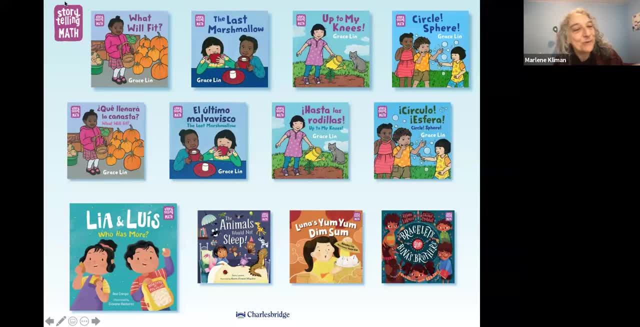 saying, just like you read to your baby from day one or before you even give birth, It's important to have those math conversations too. Yes, math conversations and diversity. I mean, obviously, Marlene is the math, and I'm going to keep pounding in the diversity thing because we have found 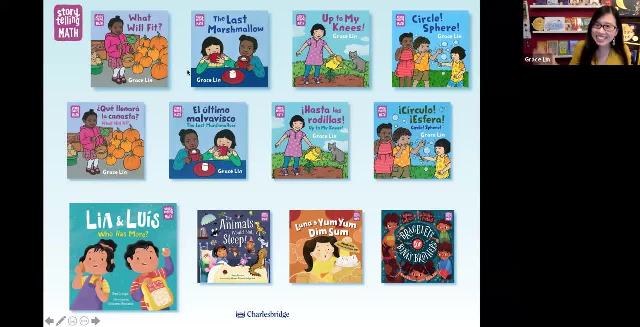 that not me personally, but studies have found that kids actually form ideas about race really early on, as early as preschool, And so for many like I live in Western Massachusetts, It's 80% white here, And so for kids who may not live in a population of a diverse population, who may not see a lot of races, 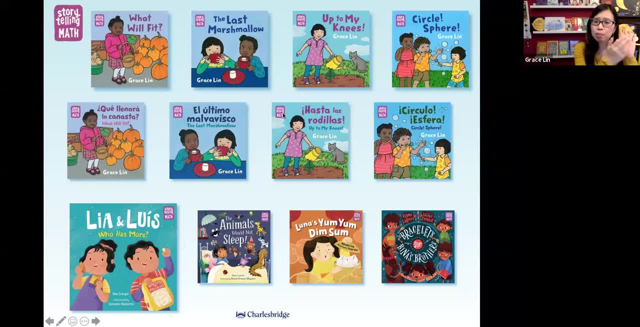 around them. it's so important to show that in books, You know like. it's not a substitute, but it's at least a first step to show them. you know the world is populated with people that either look like you or don't look like you. you know, like. 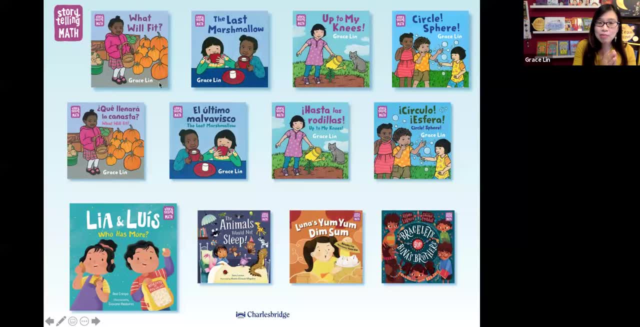 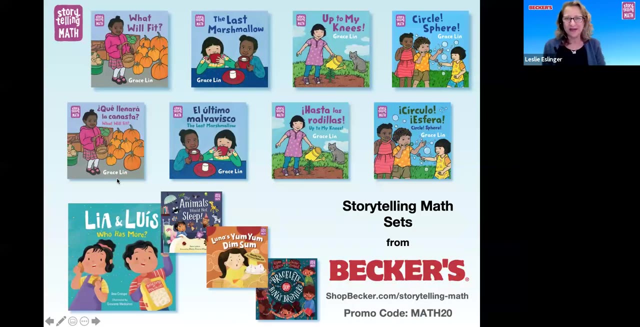 there's a global majority out there that might not be exactly the same as the population that surrounds you. I'm just looking at the time. Thank you, Grace, And I just want to start to wrap. I know that the people that are on some of their children are probably waking up from nap soon, So 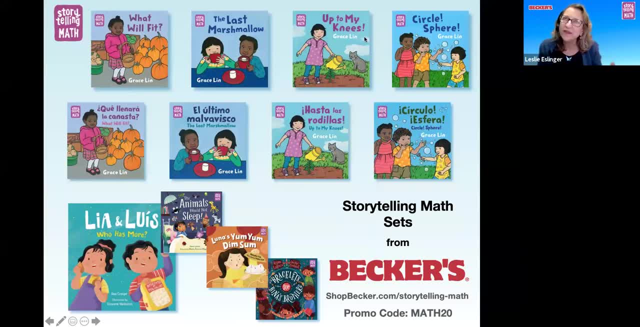 just a huge thank you to all of you. Thank you, Thank you. I think we delivered on what we promised, which was really passionate presenters And- and I think, to our presenters, we delivered a very kind audience just by reading. 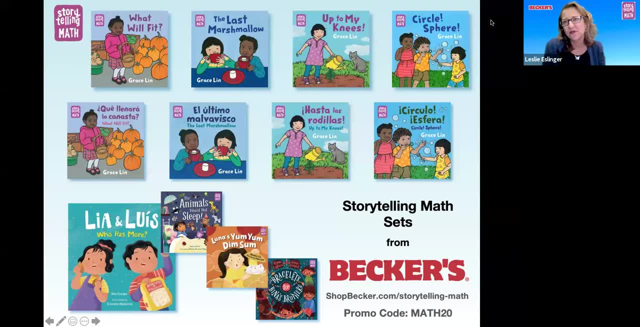 the chat. They were so engaged. I think they were so thrilled to see that we have put these kinds of materials on the market And now to fully understand what's behind it. I mean, I think, as Grace said during our practice session, you know my book is only six pages long or whatever. 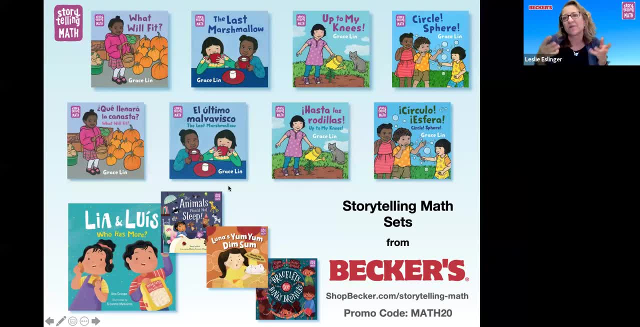 the book is, but it's packed with so much thought and clear, clear intentions of what what they wanted to communicate. So a huge thank you to everyone. I want to let everybody know you're welcome to still write in the chat. We fully understand if you need to drop off these, as I 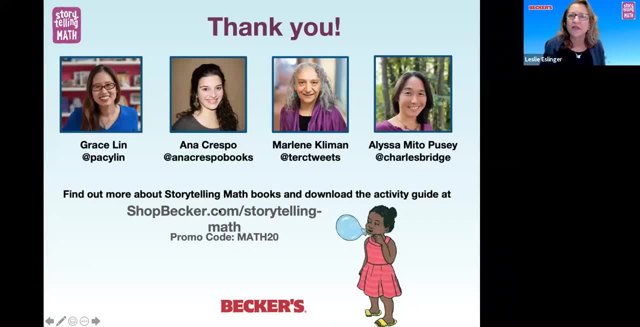 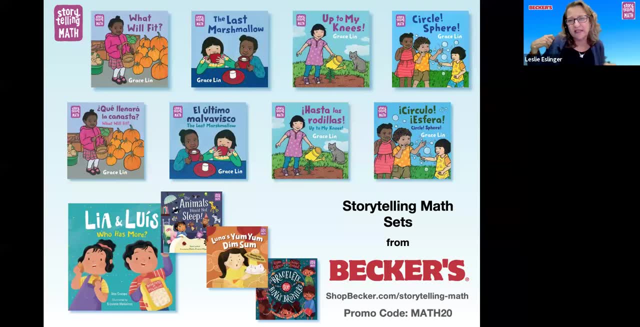 think our folks Marilyn and Terry were chatting along that everything is available, including additional resources. We will soon have the recording posted as well at this link, the shopbeckercom Storytelling math, And we do have a promo code for you. We really would love to to help you bring. 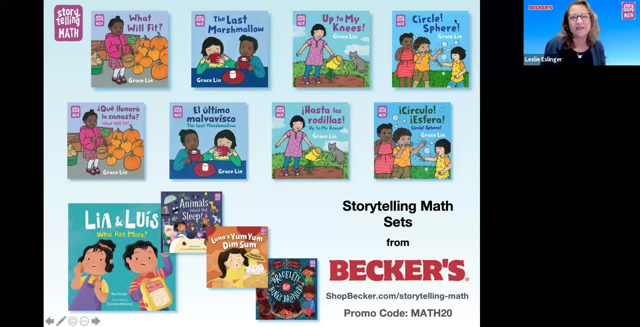 these books into your classrooms. We know budgets are tight. These books are are very reasonably priced And we- and on top of that we- just kind of couldn't help but give you an additional prompt to hope that you will make it to our website and place your orders, just to let you know the Spanish. 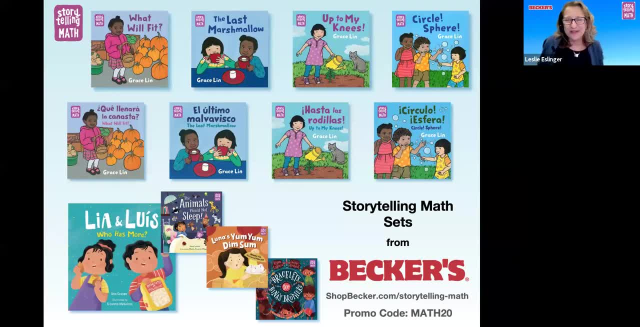 versions And I'm not sure if we have an update from the editor here, but they were a bit delayed because just all the supplies have been delayed- the supply chain situation- but you can order them now. The- the board books are all available. The. the books that Anna wrote, Leah and Luis, and the. 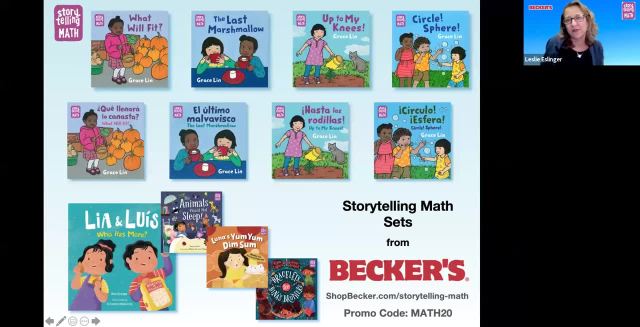 rest of that- paperback books are available as well, So we encourage you to to bring them into your classrooms and and get these messages out, which are just so all important. If anybody has additional questions for our presenters, please feel free. 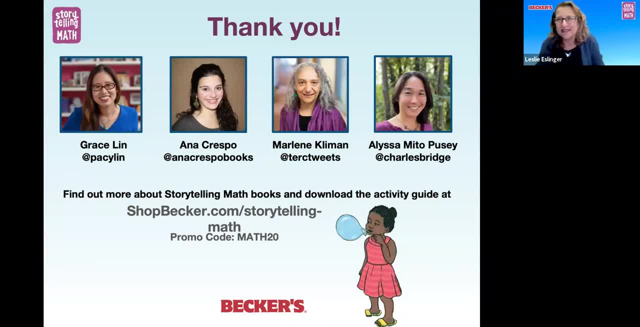 I think I kind of warned them that we might have to hang in a little later longer because our engaged- and I can see- I'm looking at the numbers- There's still so many people signed on that are just not ready to leave yet. So if you do have questions, we could try to adjust them in the 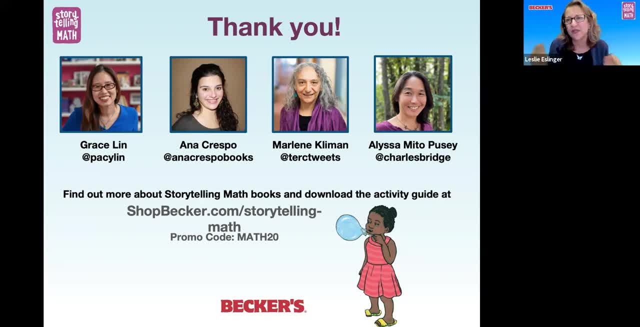 in the question and answer box, but just a huge thank you to everyone It. I even saw somebody said like they were almost moved to tears and and and I've read a lot of chats and chat boxes, but my favorite one I think so far. somebody said: 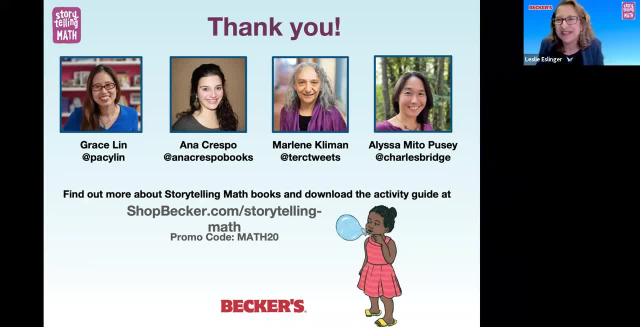 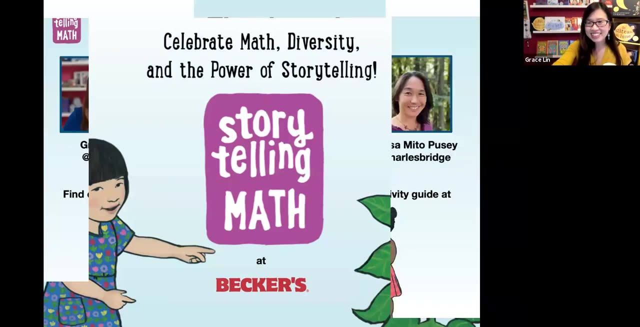 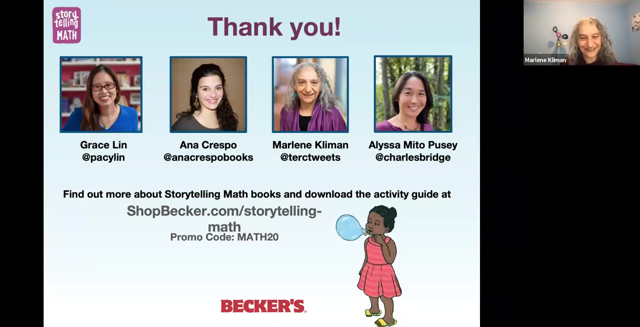 take my money. there should be more books like this, So I I just think it's a win-win for everybody. So many many thanks for being here. Yes, Thanks, so much everyone. Thank you, Thank you, Thank you for coming up with these amazing books. Oh, for all the collaboration. 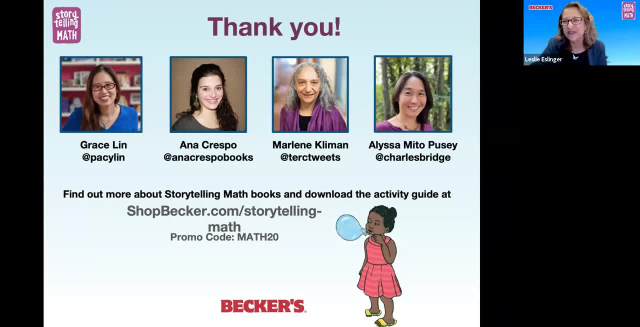 So please, authors and panelists, please leave a comment And I'll be happy to answer any questions. please read the chats. i mean, i just really want you to share in all the appreciation you're getting. i promised you a great audience and i'm telling you, becker's always has a great audience, oh and. 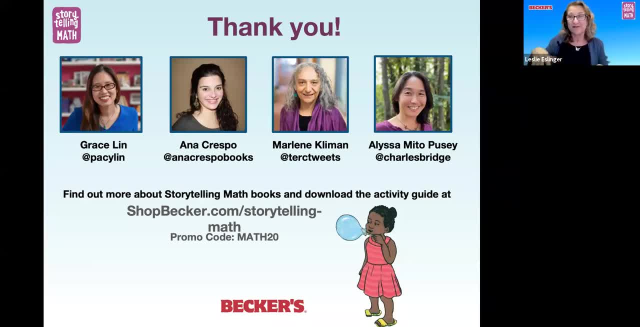 i really was going to make another announcement, because i know we have some loyalists that that file follow our webinars and we do have another one coming up. uh, december, oh december, somebody's gonna help me- december 15th, i think it is, and it is called: uh, hold on. 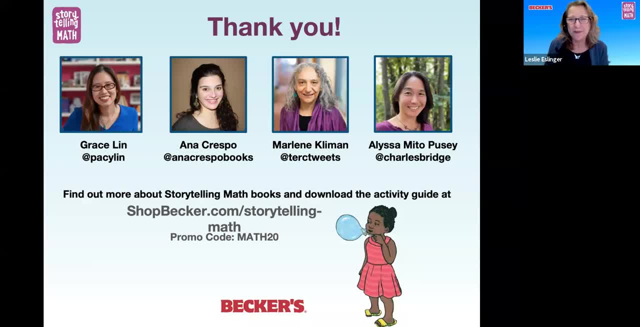 make every pose count, and it's a yoga workshop about integrating yoga into your curriculum, so i think we have a link for that as well. so anybody that loves to follow our webinars, please don't miss that one coming up next. i'm going to take my video off and just enjoy the chat box. you.